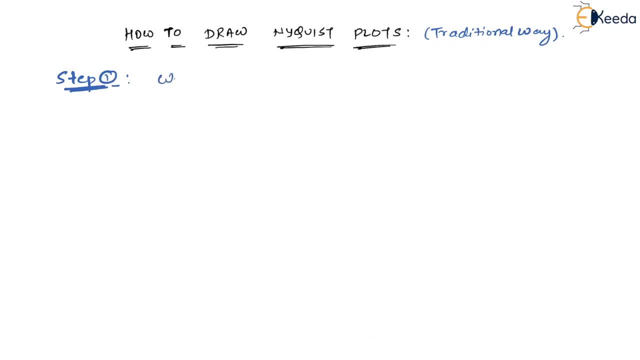 The first step is write down the open loop poles and open loop zeros, Suppose in S plane. this is the first step. It is a very easy step, right? It is nothing but our pole zero plot, only Simple pole zero plot. 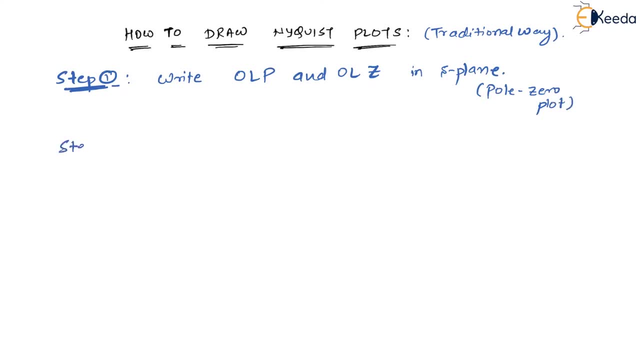 Right, Step number one. Step number two is what? Yes, Step number two is what. In step number two you have to cover. What did I say? Cover Entire Right half Of S plane. How sir? 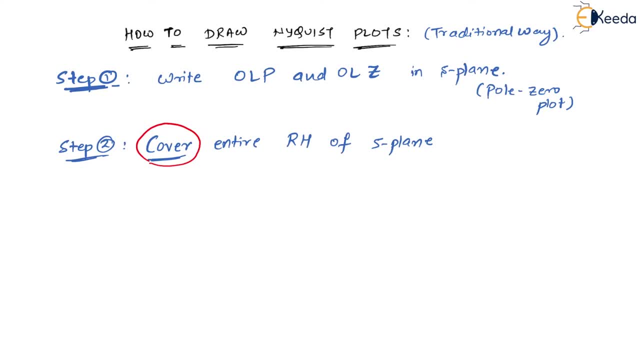 So, yes, How to cover? You have to draw. You have to draw a circle of infinite radius. How that has to be done, I will tell you, Don't worry about it, Right? This is the second step. In the second step, only in the second step only, you have to write a note. 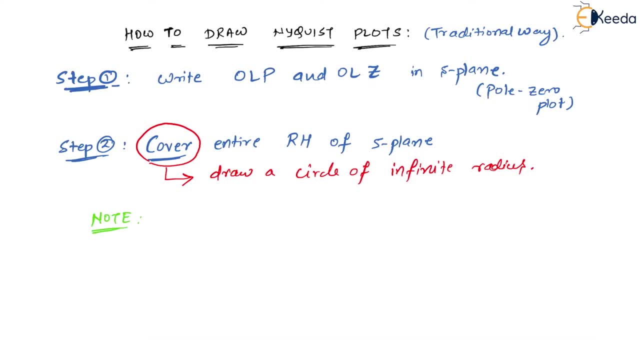 What is that note? Note is that you have to bypass pole or zero at origin. What do you mean by that? I will tell you that, Don't worry, We will take n number of examples on this. Okay, Yes, And the step three is what? 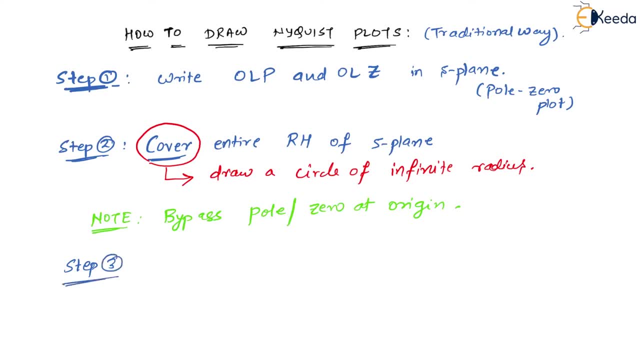 Step three, It is map the contour on g-s plane. First of all student ask me, sir, What is the meaning of contour? Contour is what? What you did just now? What did you do? You covered the entire right hand side of the s plane, right? 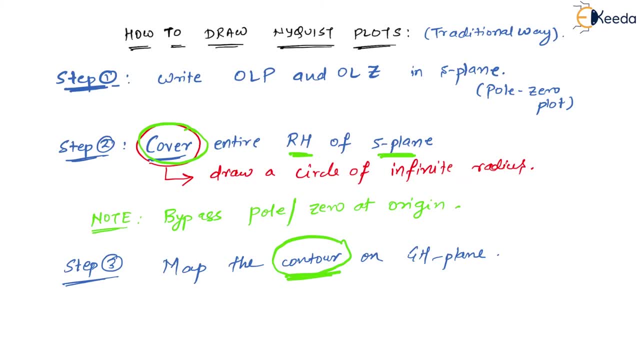 That is nothing but contour. So from s plane now, if you see, you have drawn it on the s plane right. So from s plane you have to map it to something called as g-h plane. What is that? 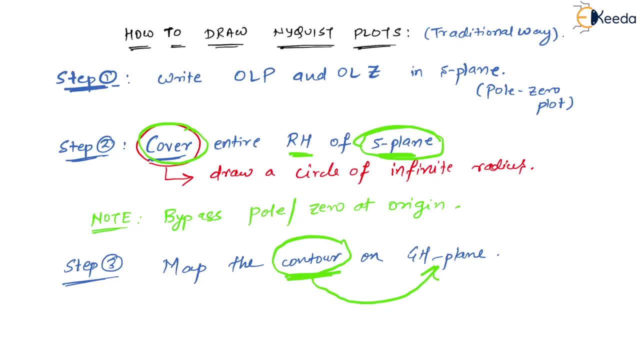 I will tell you that, Don't worry, It is going to be very, very easy. If you remember, on g-h plane we had also plotted something else, And that something else was polar plot. Right, Yes, Okay, So now. 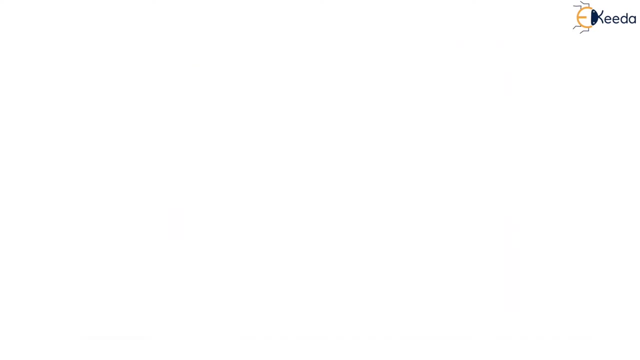 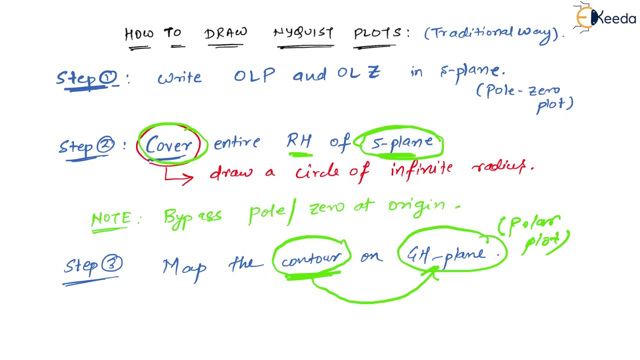 Starting with the first example. if you see, Let us begin. Let me take the first example. See, dear, If you see before that example, Let me just ensure you about one thing. You may ask me, sir: Why are we interested in the right hand side of s plane? 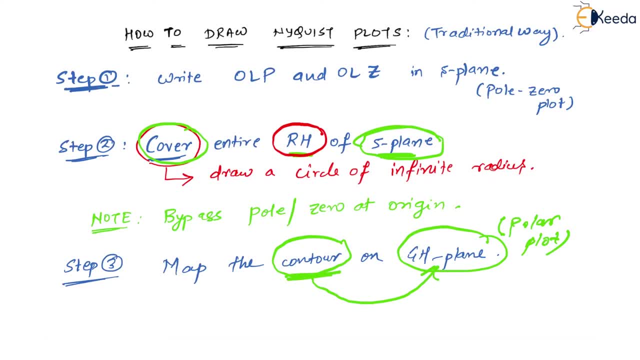 Why? Because If you know That Right hand side only gives you Unstability. If you remember Right, If you remember Poles on the right hand side of the s plane Always gives you instability. So we are interested into the right half of the s plane. 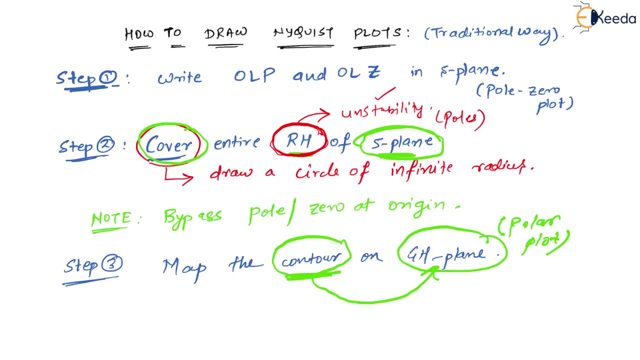 This is the reason, Because we have to check Whether there is any pole there or not. How to check that on all, We will talk about that later, But for time being it is okay. Right, Let us take the first example. 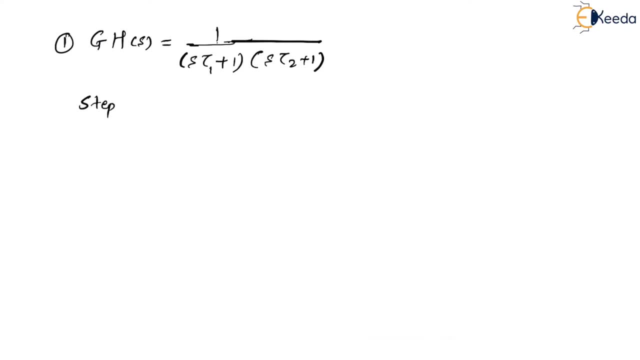 Yes, Step 1 is what? Step 1 is very simple. Step 1, if you remember, It was just to draw a pole zero plot. Let me draw a pole zero plot, Step 1.. So pole zero plot is what? 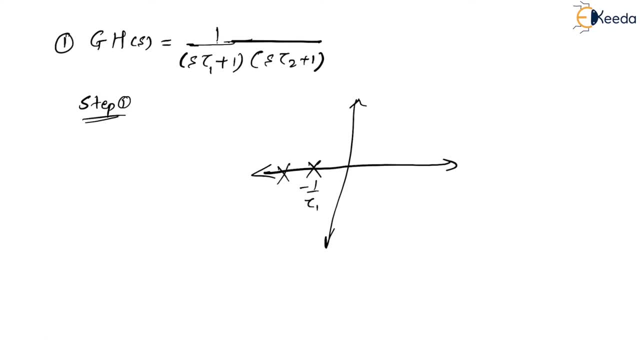 Yes, It is going to be minus 1 by tau 1.. This is one pole, and another pole is minus 1 by tau 2.. See If you equate. If you equate this one to 0. What you get is tau 1 plus 1 equal to 0.. 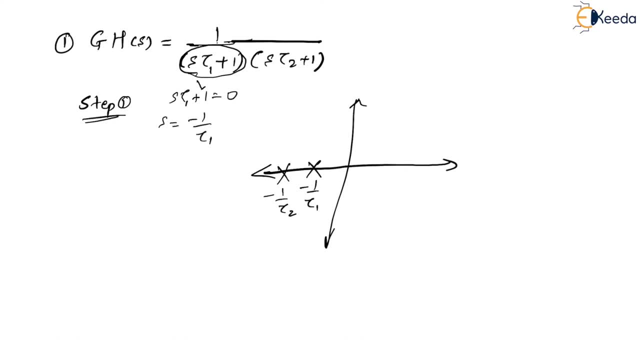 So you get s equal to minus 1 by tau 1.. Similarly, if you try this out here also, So you will get that particular pole to be minus 1 by tau 2.. Yes, Definitely. So the pole zero plot is available now. 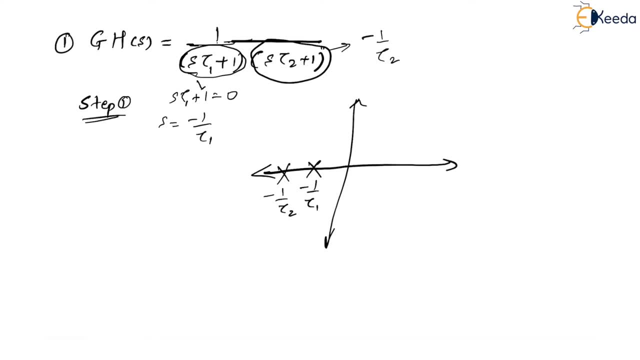 Ready? Now the next step. What are we supposed to do? Let me do the step 2 here itself. Let me tell you how. If you remember, This is going to be S plane, This is s plane, So in s plane. 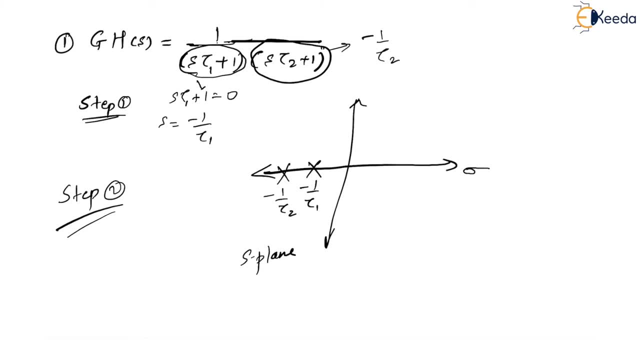 Here on the x axis, we have sigma, Which is the real part of the s plane, And we have here imaginary part of s plane, Which is nothing but j omega, if you remember. Yes, Now I want to tell you some things. 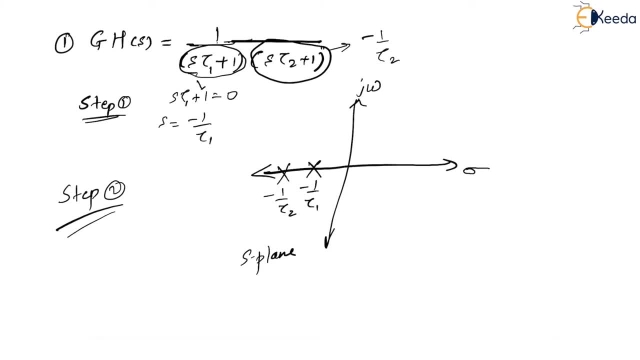 Which are very, very important. See, If you see, Do you agree with me that this particular y axis Represents omega? Yes, It shows you omega. And here, on the down side, if you see, If you just go below, below, below, more below, 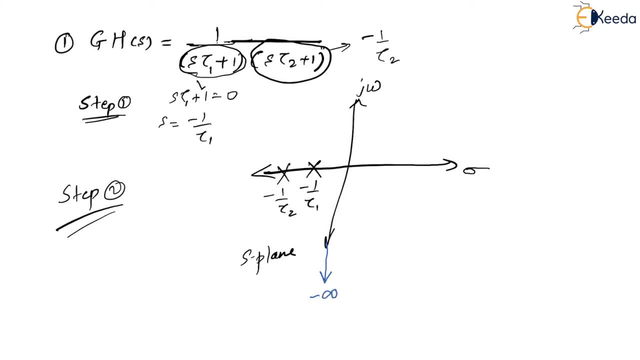 You get minus infinity, right? Omega equal to minus infinity. Yes, This is omega equal to minus infinity. Similarly, if you go on the top, top, top, So what you get here, You get omega equal to plus infinity. Is that correct? 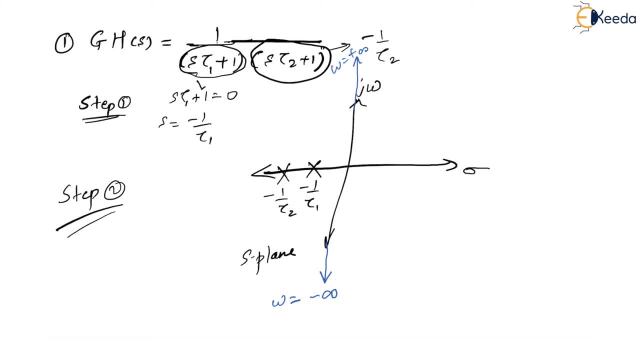 Yes, It is correct Right Now. What am I interested in? I have to cover the entire s plane Right, half of the s plane Right, half of s plane Right. So, in order to do so, What will I do? 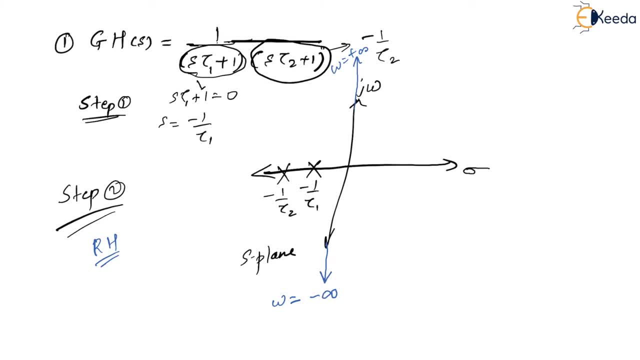 Let us see. In order to do so, What will I do? Let me tell you: The first thing that I will do is I will start from minus infinity And I will move up to zero. Is that alright? I will move from minus infinity. 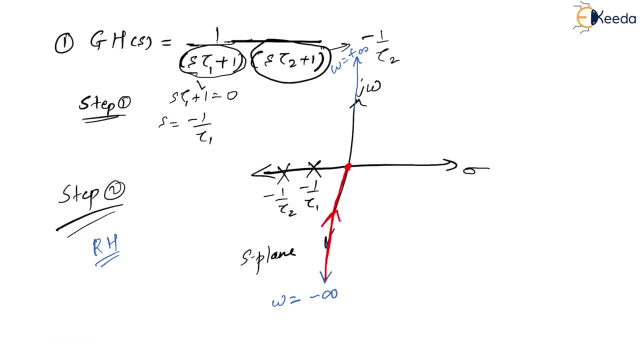 Yes, So when I move from here to here, Let me draw that this particular area, Let me call that this is Contour C1.. Contour C1.. Is that alright? So if I try to show that, 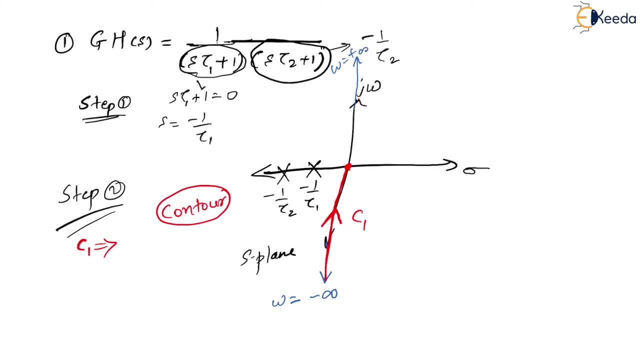 Represent you C1. Then you understand that C1 is what C1 is: from omega equal to minus infinity To omega equal to zero. Is that correct? Yes, This is your C1 contour. Right Now, Let me start moving from. 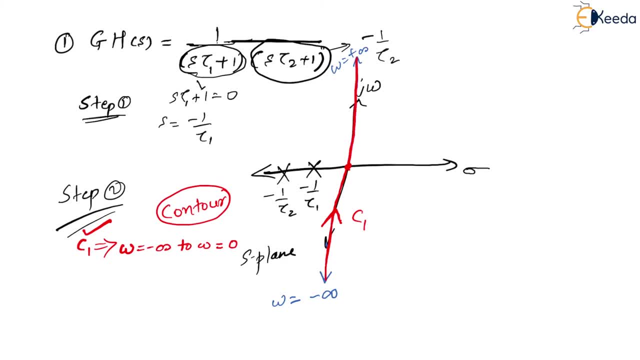 This zero To positive infinity. What do I get then? If I start from zero to positive infinity, then Then this particular contour, Let me call this contour as C2. And this is Heading up to Infinity Right. So if you think of 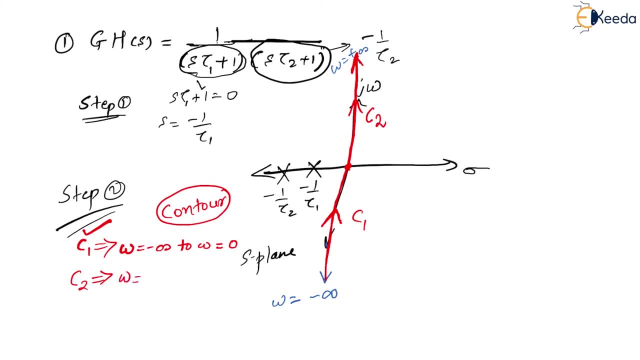 What is my C2?? C2 contour is what C2 contour is. nothing but Omega Varies from where to where. At origin, it is zero To omega, equal to infinity. Is that right? Yes, Now This is my entire imaginary axis. 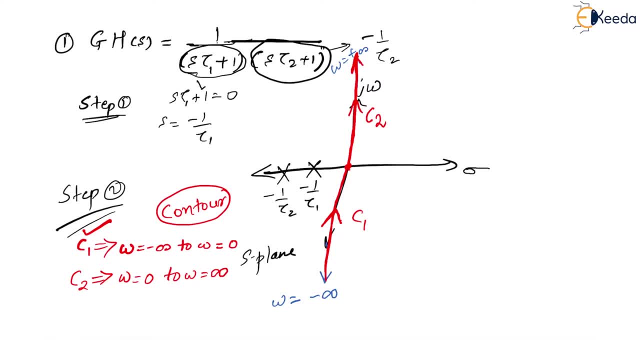 C1 and C2.. Shows you that Now. But you are interested in what You are interested in: entire Right half of the S plane. So, since you are interested in Entire right half of S plane, What will I do is? 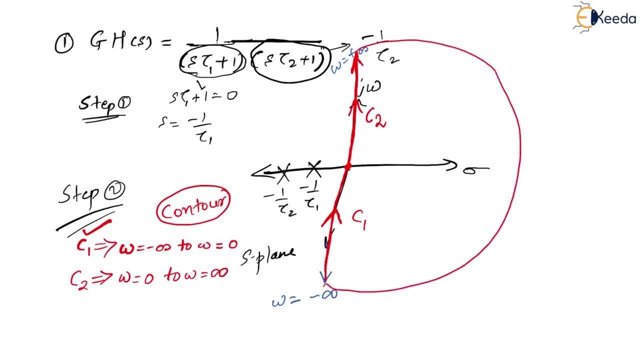 I will draw a infinite radius circle Over here. What did I say? I will draw a infinite radius circle Over here, My entire, Such that my entire Right half of S plane Is covered. Is that correct? Yes, Now see here. 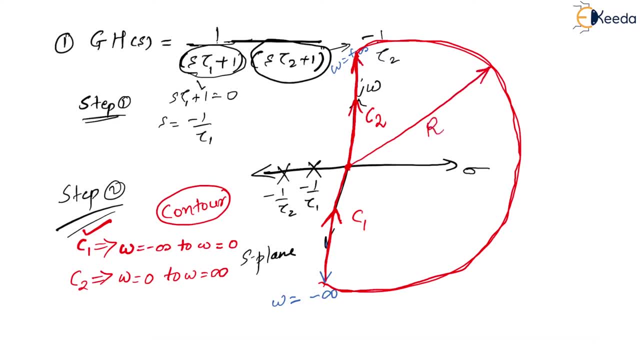 What did I say? This is infinite radius, So let me just mark the radius to be infinite. So this is radius R, Which tends to infinity. Is that correct? Yes, Now See here, If you remember, You have studied. 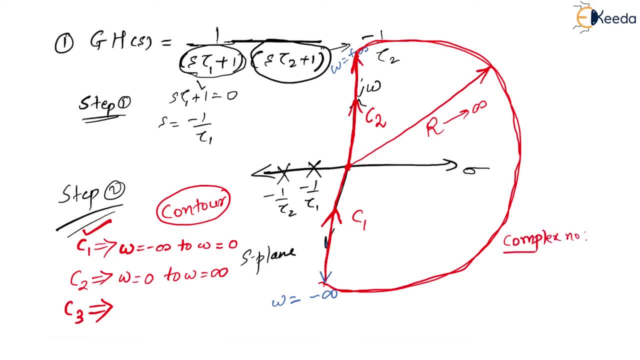 Something called as complex numbers Right There, you must be aware of That a particular complex number, Because see this particular S plane Right, This is all S plane. So if you see that in this S plane also, You have something real part. 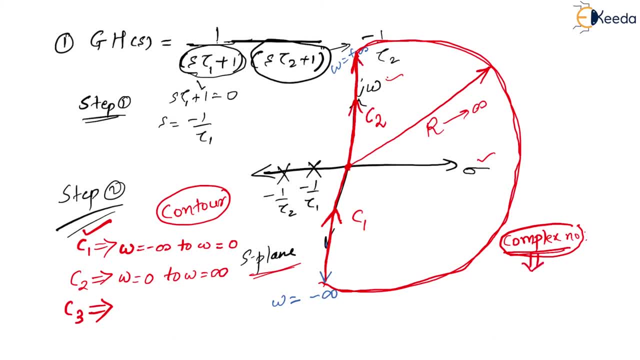 As well as some imaginary part Right. So there you have seen that Can be represented In the form of exponential, In the exponential form Right, And that exponential form was Z equal to R into e, to the power I theta. 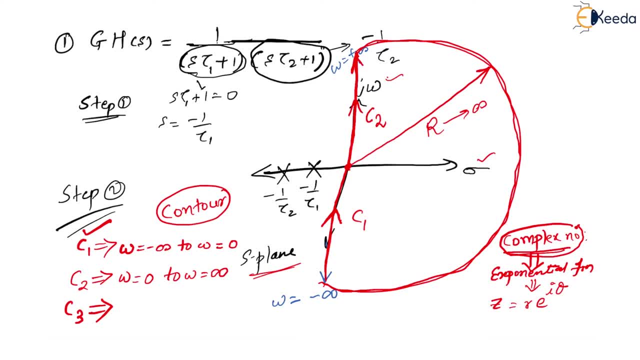 Right, Yes, Similarly so. in order to show This particular circle, This particular circle, What will I do is I will put It by R into e to the power J theta, Is that correct? Why? Because I am saying that 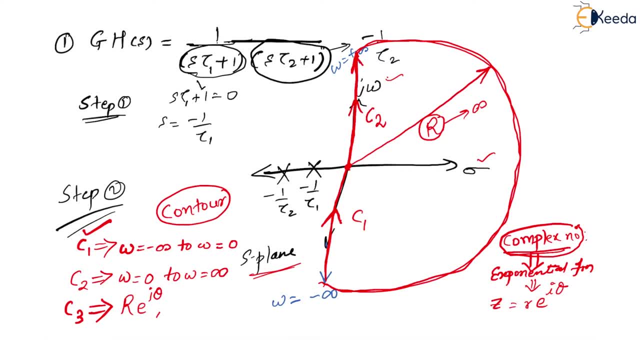 This capital, R is the radius of this circle. I know it is going to infinity. So with this C3, if you see It is what It is- R into, e to the power, j theta, With R moving towards infinity, And if you think of this theta, 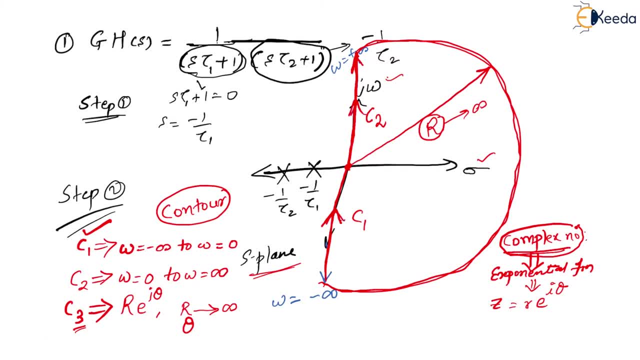 What is this theta? then We have gone this way: So this is C1.. This is C2.. So this becomes your C3.. So if you see, We are going from, We are going in this direction, Is that right? 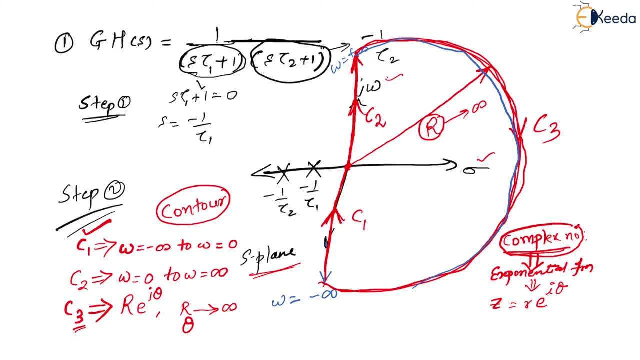 Let me show it with another color. So if you see, We are moving in this direction, This direction, This direction, Which means Theta goes from. So if you see, I am moving from plus 90 to 0.. 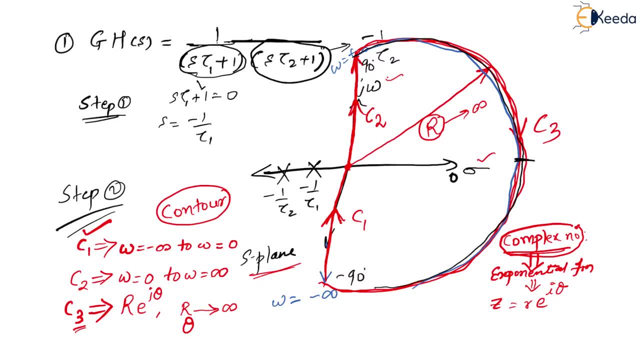 To minus 90 degrees, Which means theta goes from where to where Theta goes. from where to where Theta goes from Minus 90 degrees to 0. To Sorry: Positive 90 degrees to 0.. To minus 90 degrees. 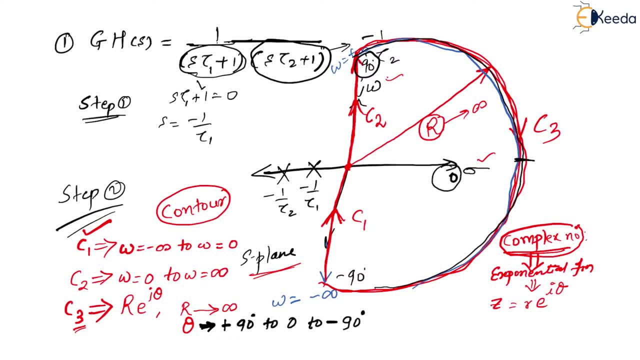 Is that right, Because this is plus 90. Then we went up to 0. So this was our whole journey Of the circle Right. So here, if you see, Now you have this entire Entire right half of the S plane. 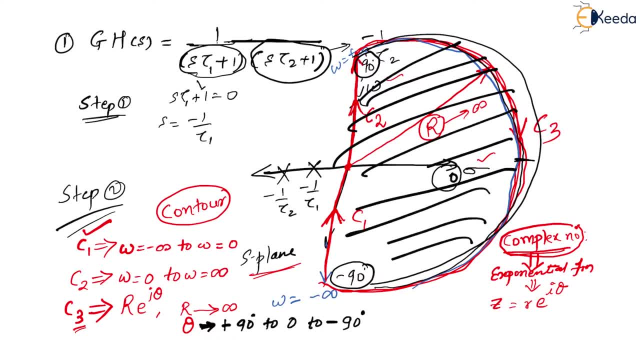 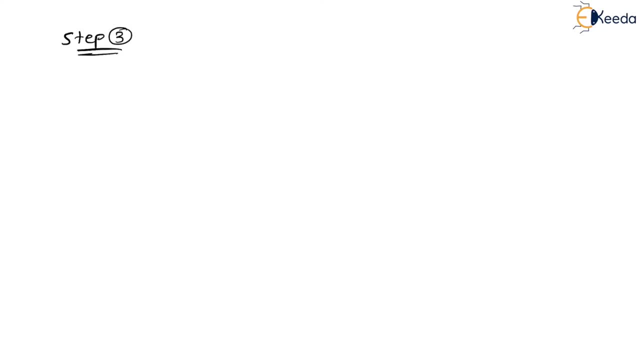 Along with the imaginary axis In your, In your scrutiny, In your scrutiny. Is that correct? Yes, Now step 3.. What is step 3, dear? Step 3 is what Map? Contour to GS plane. Contour to GS plane. 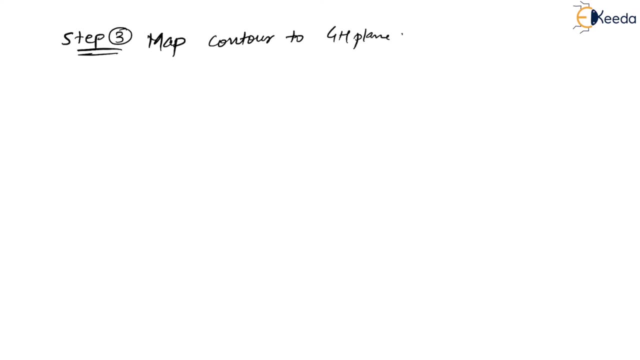 Contour to GS plane. How to do that mapping? Let us see. Let me firstly draw this contours. How are those contours? if you see? Let me draw it here For simplicity. If you see, this was the S plane, This was sigma. 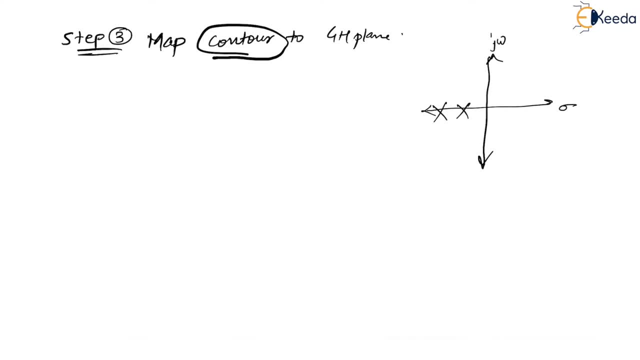 This was j omega Right Now. If you check out, Here was omega equal to minus infinity And here was omega equal to infinity. So we have started from here to here. We went up to 0.. So this was C1.. 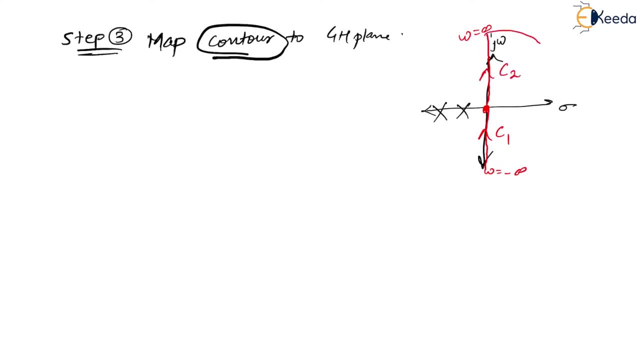 Then again, we started from C1. We went up to infinity, So this became C2. Right, And then we just closed it. We just closed it this way. Right, It is from omega equal to minus infinity To 0.. 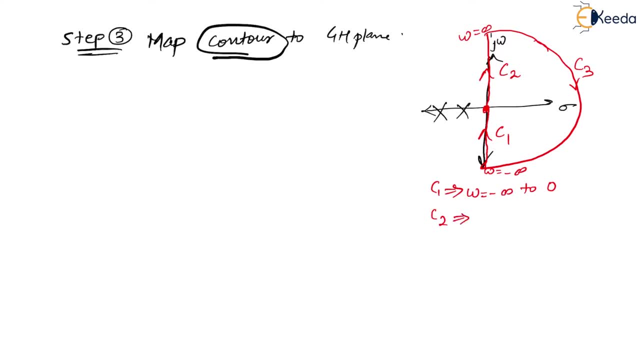 Then what is C2?? C2, if you see, It is starting at 0. And it is ending at omega equal to infinity. So it is omega equal to 0 to infinity. And if you think of C3.. C3 is what? 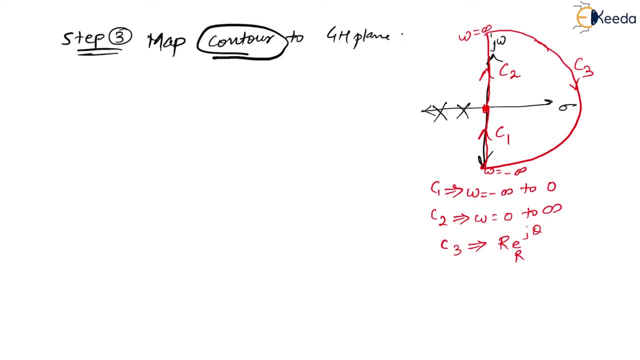 C3 is nothing but R, e to the power j theta, Where R is moving to infinity And your theta Theta is moving from where to where? From this point To 0.. To minus 90 degrees. Is that correct? 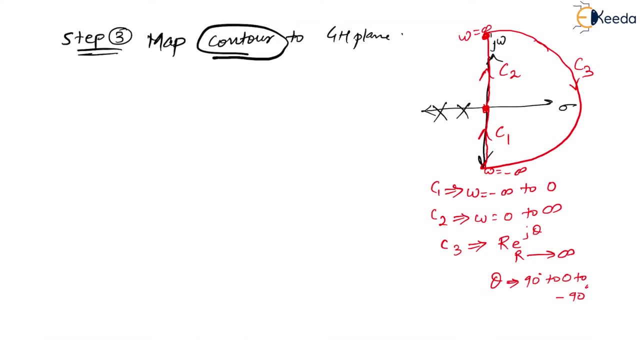 Yes, Now let us draw the Nyquist plot. Let us see that. Let me call this plane as GH plane. So here I will be having real part of GH, As we already know, And here I will be having Imaginary part of GH. 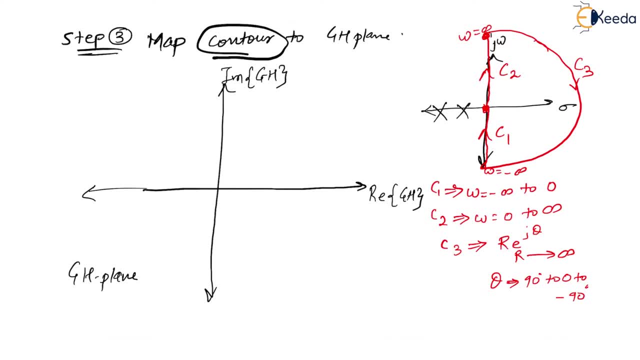 Is that correct? Yes, If you observe C2 contour is what C2 contour is, from omega equal to 0 to infinity. If you remember, Omega equal to 0 to infinity is what It is, nothing but Polar plot itself. 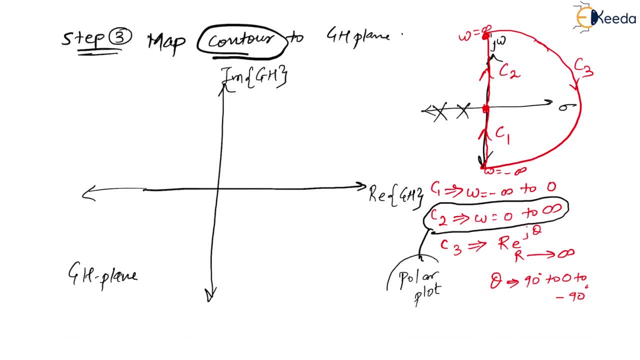 Polar plot itself. Right, Because we know that It is the variation of magnitudes and angles With respect to omega, Which is varying from 0 to infinity. I hope you are aware about this. We have talked about it a lot. 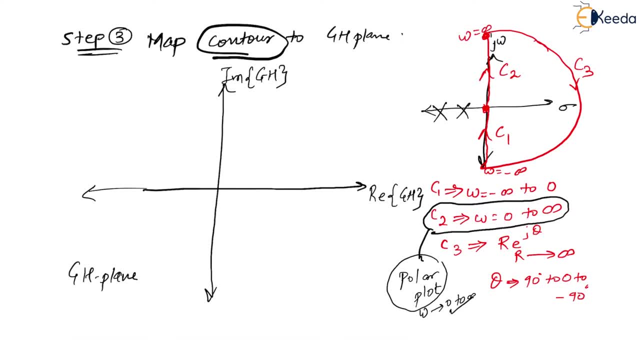 Right, We have done Total 5 parts on that, Right. So if you think of That, this one is the plot. So From the shortcuts You can say that This particular plot or, If I may, just You know, start with it. 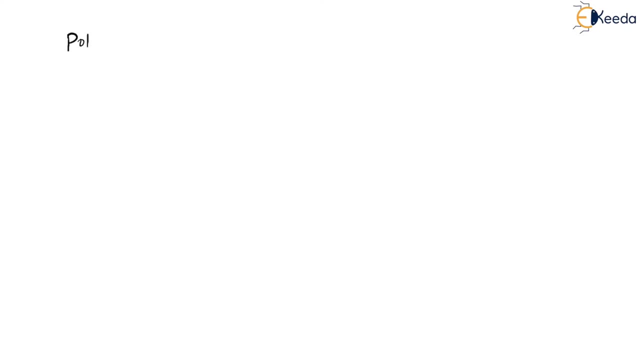 Let us try to See those specifications for the polar plot. How to draw the polar plot? We had the four step method. What was that method? Step 1 was what. Step 1 was to find M0 and M, infinity and all. 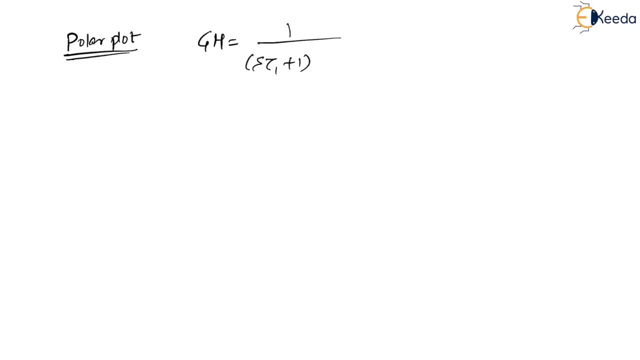 But then what you have is You have gh which is equal to 1 upon s tau 1 plus 1.. Into s tau 2 plus 1.. Right, So you are interested in gh of j omega. Right, If you think of gh of j omega. 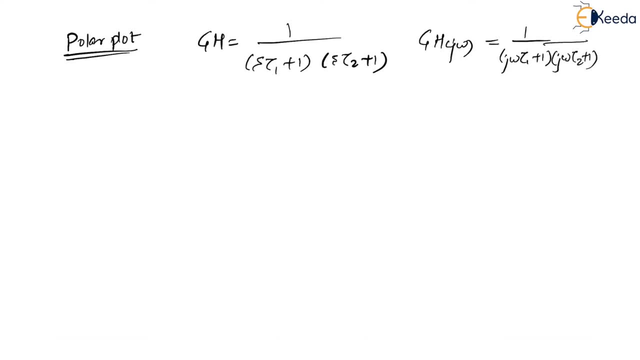 It becomes 1 upon j omega tau 1 plus 1.. Into j omega tau 2 plus 1.. Is that correct? If you think of the magnitude, How much is the magnitude? How much is the magnitude? It is nothing but 1 upon. 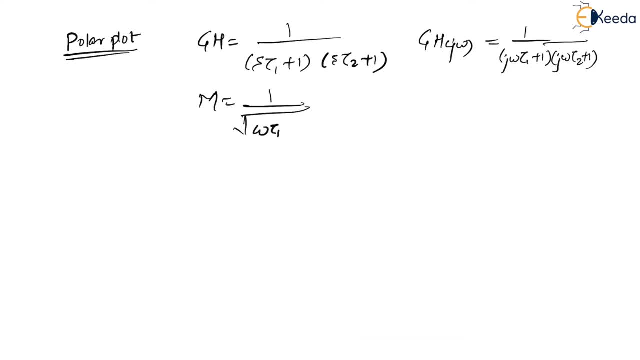 Under root of Real part squared plus imaginary part squared, So it becomes omega squared, tau 1 squared Plus 1.. Right Into what does that become? Under root of omega squared, tau 2 squared Plus 1.. Is that correct? 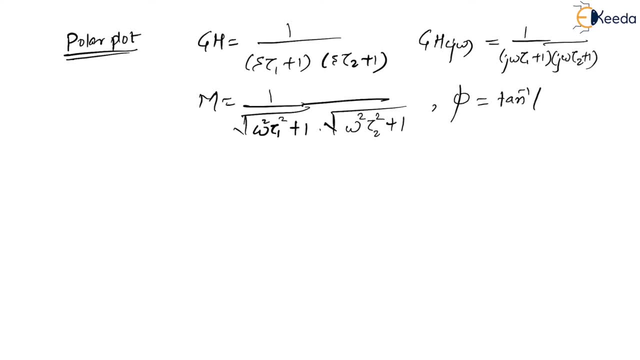 Yes. Similarly, if you think of phase 10, inverse of what? Omega tau 1 by 1.. Right Minus 10 inverse of Minus, Again, you have this: 10 inverse of omega tau 2 by 1.. 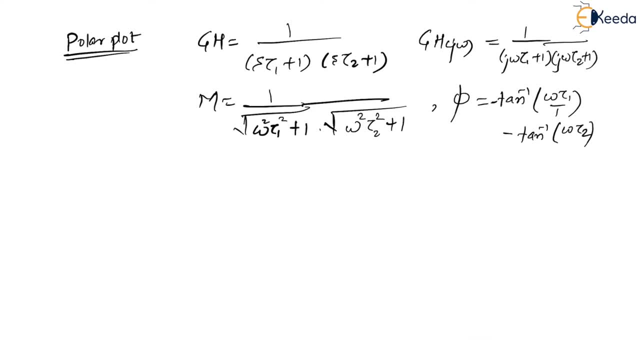 Is that correct? Yes, See. So, if you see, We have talked about it a lot. So this is for the first and last time I will be explaining you, Because we have dealt about it A lot in our previous sessions. 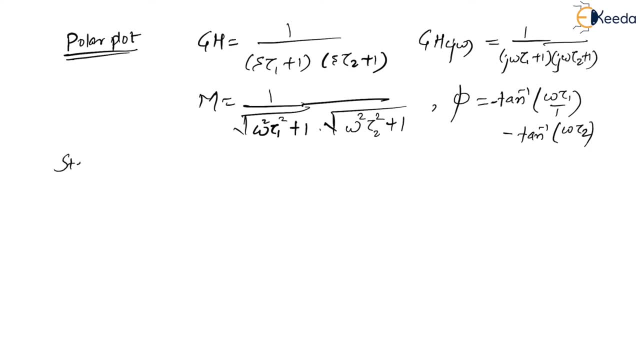 Right, Yes, So now the step 1.. Step 1 is what? Step 1 is nothing but to find M0.. How do you find M0? M0 is what Magnitude at omega equal to 0.. How is it? 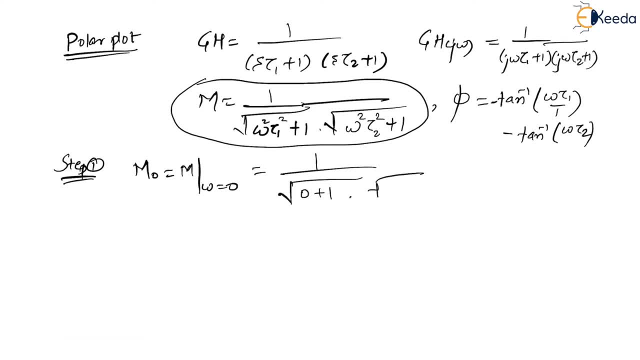 It is nothing. but what If you just replace here by omega In this magnitude, What 1.. So M0 is equal to 1. What about M infinity? M infinity is nothing but magnitude at omega. equal to infinity. Which is equal to what? 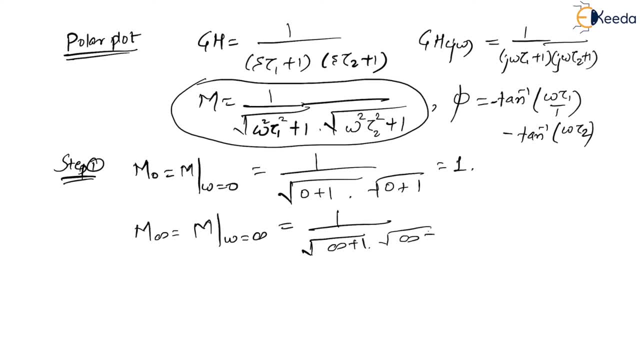 1 upon under root of. If you think of, this becomes infinity. Into again infinity plus 1.. Infinity plus 1.. So this is nothing but 0. Is that correct Right Now, if you think of step 2.. 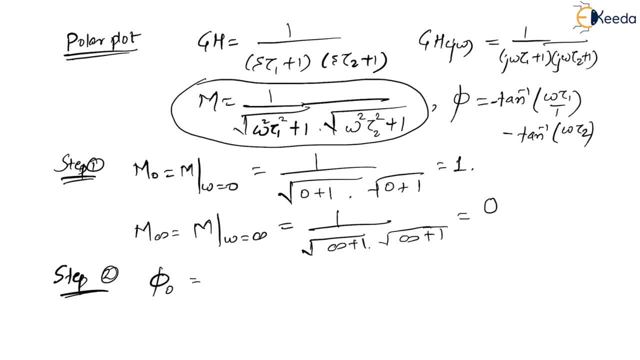 What was your step 2?? M infinity and M infinity. What is M0, dear M0 is what M at omega equal to 0.. Which is equal to what Minus tan inverse of 0.. Minus tan inverse of 0. 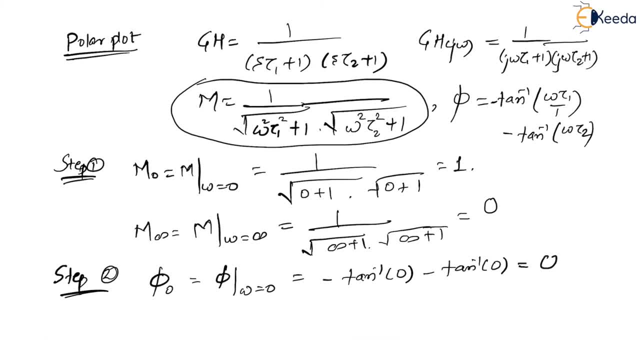 Which is equal to what? Which is equal to 0.. Right, Then, what is M infinity? M infinity is what? It is: nothing but M at omega equal to 0.. Which is equal to minus tan inverse of What do you say? 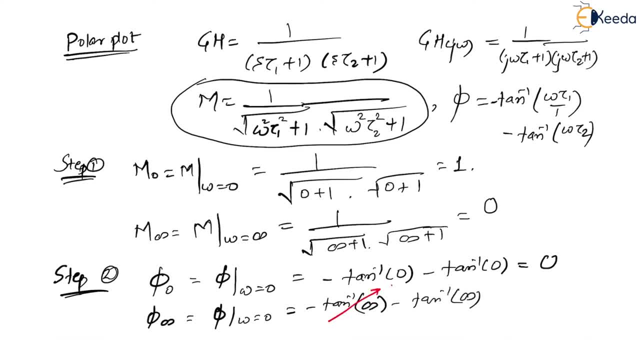 M. infinity is nothing but tan inverse of infinity. If you see, Tan inverse of infinity is 90 degrees. Tan inverse of infinity is 90 degrees. So minus 90 minus 90 you get Minus 180 degrees. Is that correct? 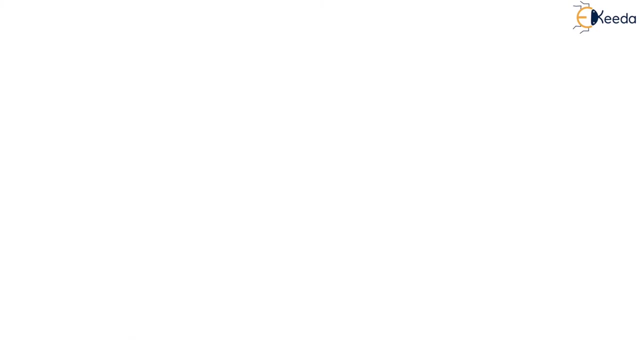 Yes, What does this mean? Now? step 3 is what. Step 3 is to find this ending direction. Right. Step 3 is what To find ending direction. What is that? 5 infinity is what Minus 180 degrees minus 0.. 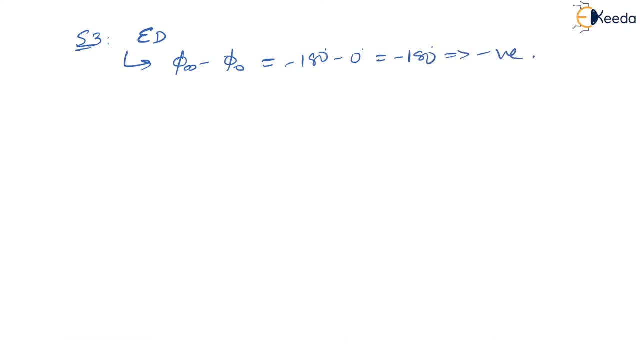 So it becomes minus 180 degrees minus 0.. Which is nothing but minus 180 degrees, Which is negative. This means that ending direction has to be, Ending direction has to be. how much Has to be Clockwise, Is that correct? 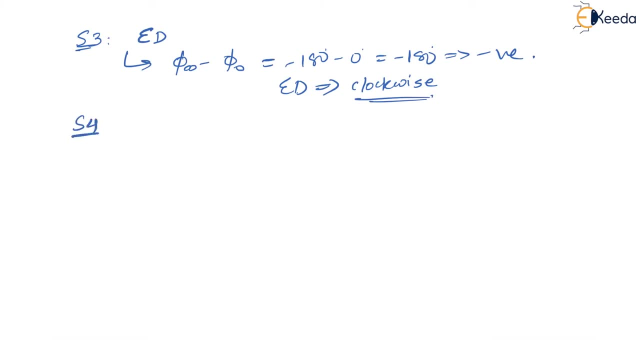 Yes, Ending direction has to be clockwise. Now, what is step 4? Starting direction. Starting direction is what? Starting direction is what? It is nothing. but You have to draw the pole 0 plot, Which is this way. You already know. 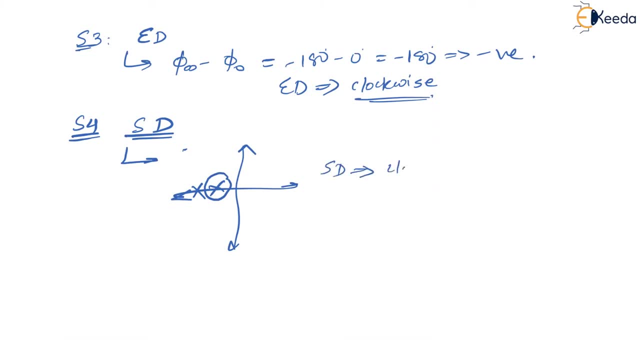 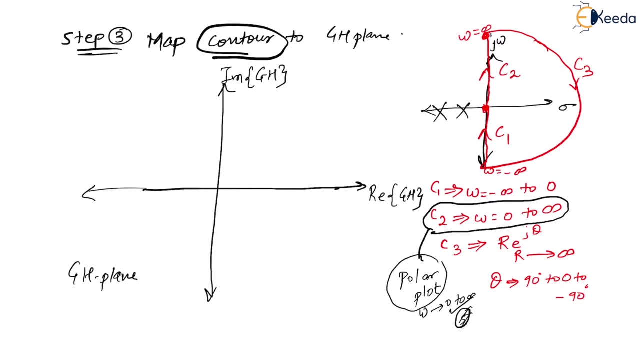 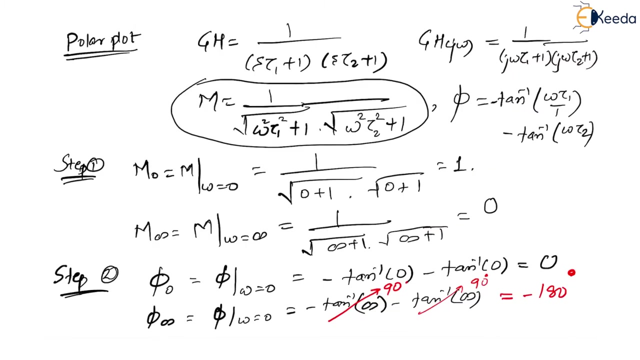 And if you see that You have this pole closer to the origin, Which means that Starting direction has to be also clockwise, Is that correct? Yes, So if you see here, Starting direction is 0. Right, Yes, How do you know that? 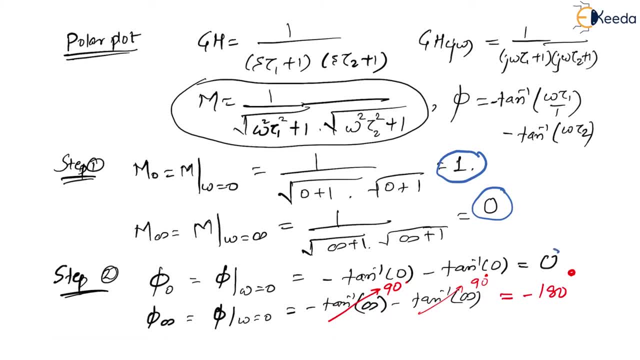 Because m0 is 1. And m at infinity is 0.. Now, angle at omega equal to 0 is 0.. Right, That is the reason It is here 1.. Now angle at omega equal to infinity is what. 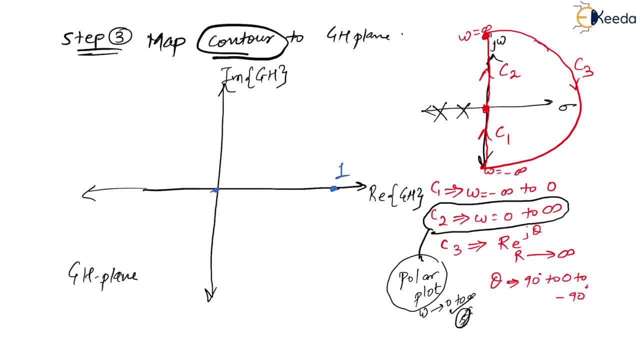 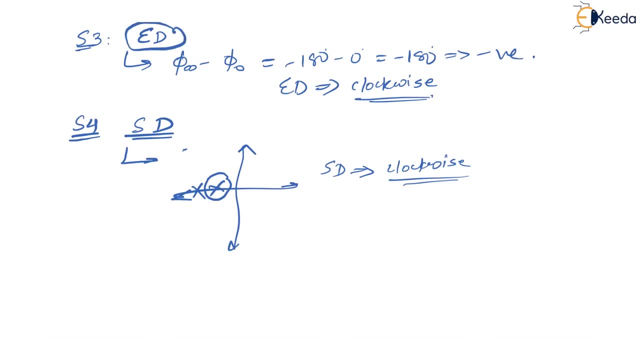 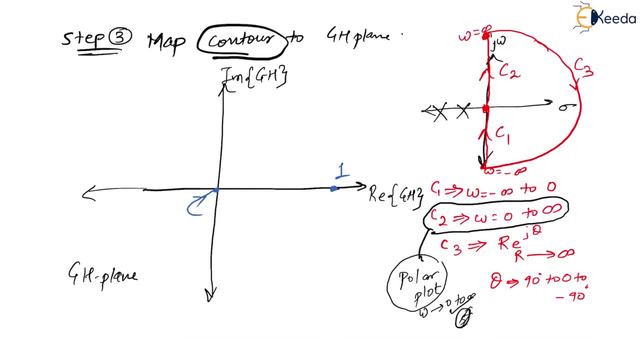 Minus 180 degrees, Which means here, Here itself. See, I will explain. you See, Ending direction is what? Ending direction is clockwise, Which means Definitely it has to move in this particular direction. Clockwise direction, Right. 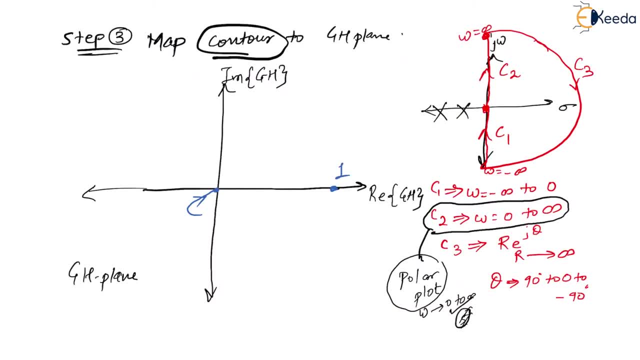 Yes, Now, If you think of starting direction, Starting direction is also what Clockwise. So, yes, This was the polar plot And if you remember, This is nothing but what. This is nothing but your contour C2.. 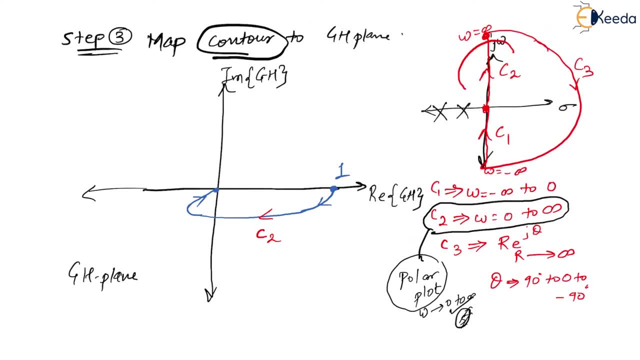 Which is mapped from this S plane, This particular contour C2.. Let me take another color: This particular contour C2.. Is mapped from S plane to GH plane. I hope it is clear to you, Right, If you see C1.. 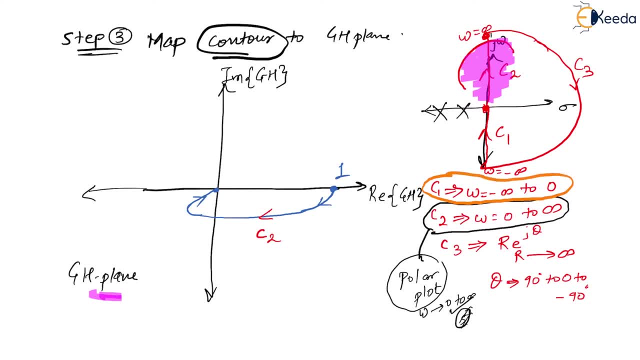 From omega equal to Minus infinity to 0.. Right Now I will tell you one thing: If you see, Here, Since it is starting, Since my plot is starting here, Which means here, omega equal to 0. Right, 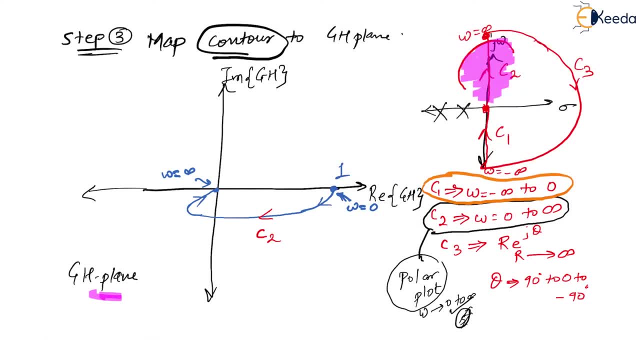 And here Omega is nothing but infinity. Right, It means that You have to take a mirror image of this Like this: So this becomes now Omega equal to minus infinity, And this becomes omega equal to 0.. Is that clear to you? 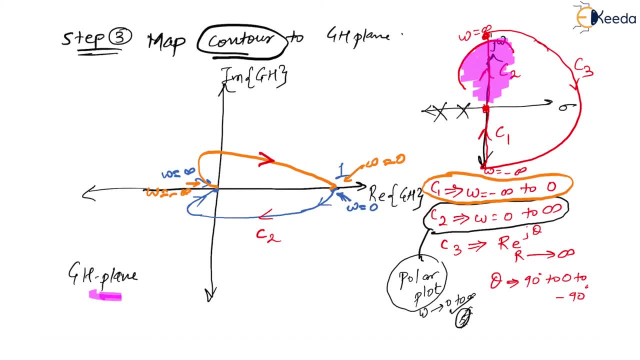 Yes, Now This is nothing but contour. This is nothing but your contour C1.. So, if you see, C1 has been drawn. Now what is being tested in mapping C3?? How to map C3? That is the question. 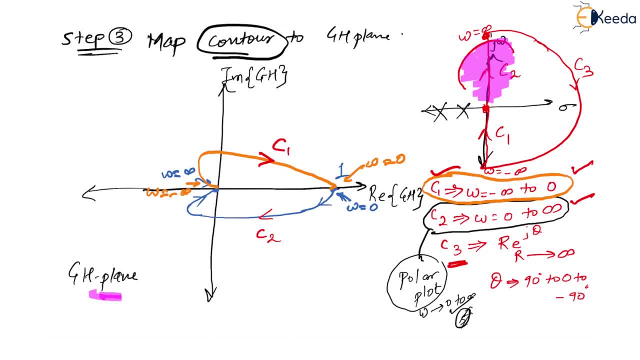 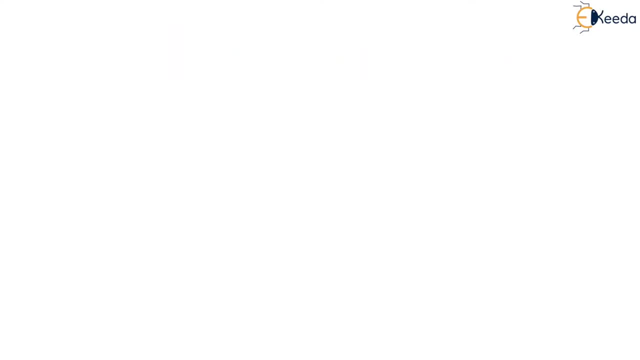 Right. So if you see It is nothing but R into e to the power j theta. So what will I do Now? see, you have to map this in what You have to map this in GH, Right? So very simple. 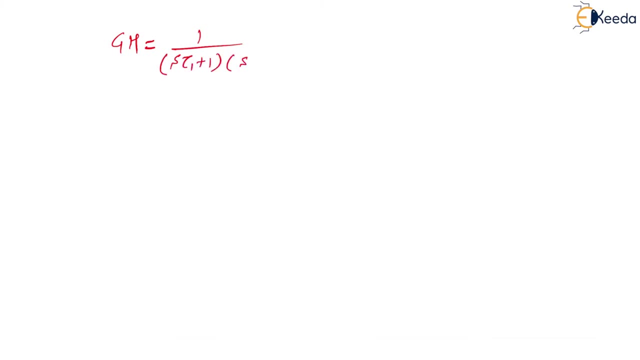 What will I do is: What is your GH, dear GH? is what 1 upon? What will I do? I know that in S plane I have a contour, Contour Which is R into e to the power j theta. 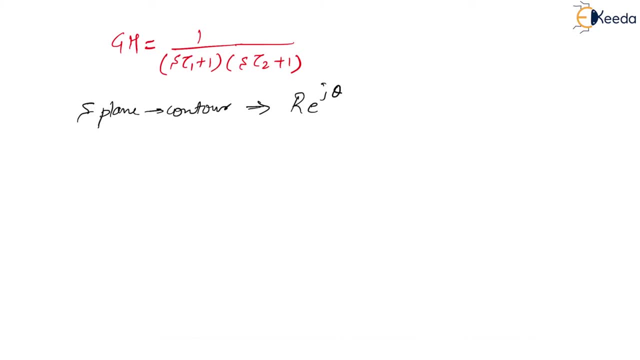 Is that correct? Yes, Now I want to map this contour Onto GH plane, So I will simply replace My S By R into e to the power j theta. So If you find GH of R into e to the power j theta. 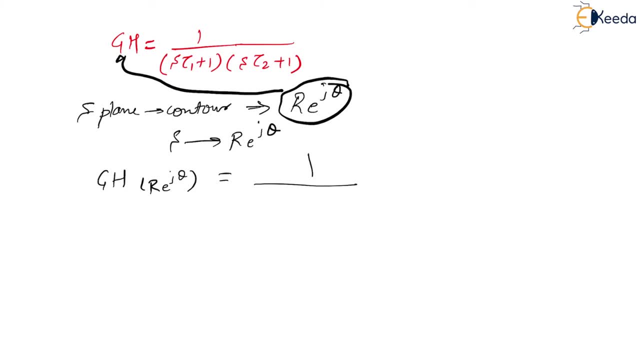 Which means, Wherever you have S, You please replace it by R into e to the power j theta. So after replacing that, you get R into e to the power j theta Into tau 1 plus 1.. Into again. 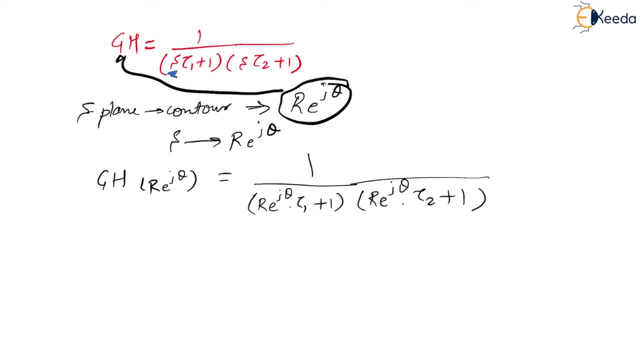 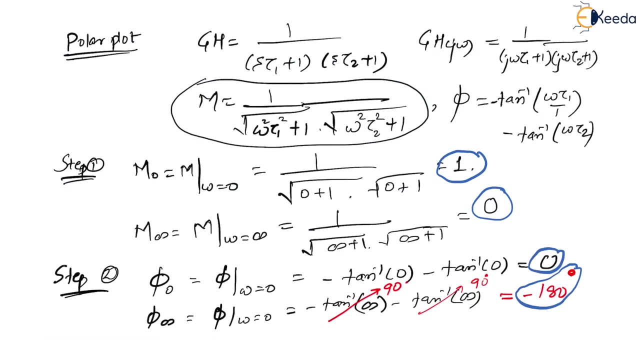 R into e to the power, j theta Into tau 2 plus 1.. Is that correct? Yes, If you see it here In place of S. Right Now, if you know, If you remember My R, Where is that? 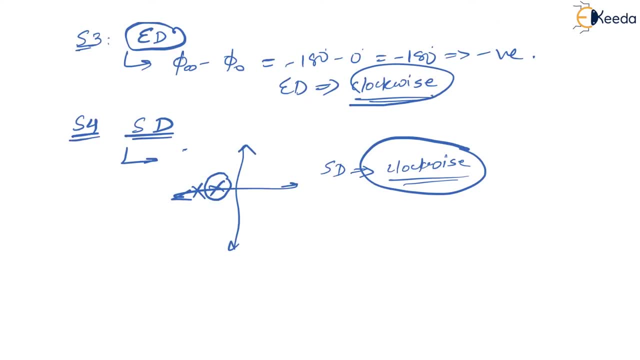 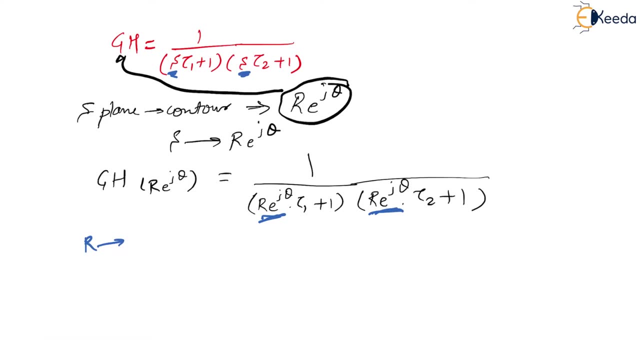 Yes, If you see, My R goes to infinity, R tends to infinity. So If my R is tending to infinity, What happens then? What happens to the magnitude? Let us understand. So: 1 by infinity into infinity. 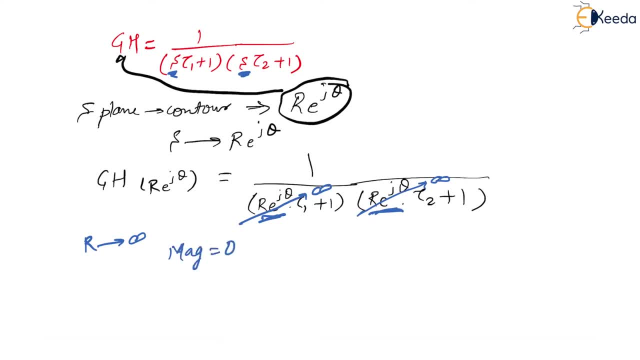 Is nothing but all 0. Which means magnitude is going to be 0.. What about angle? What about angle? If you see Angles? How was that angle? Angle was nothing but plus 90 degrees to 0.. To again minus 90 degrees. 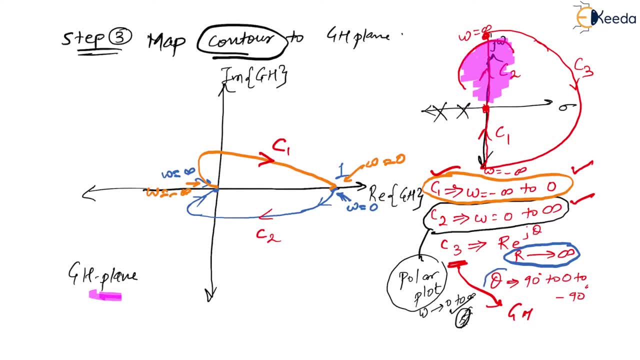 Is that right? Yes, Why? Because here we have already seen, Angle is minus 90 degrees. Yes, So what do you understand from this? You understand that Contour, Contour C3. Is mapped Because see. 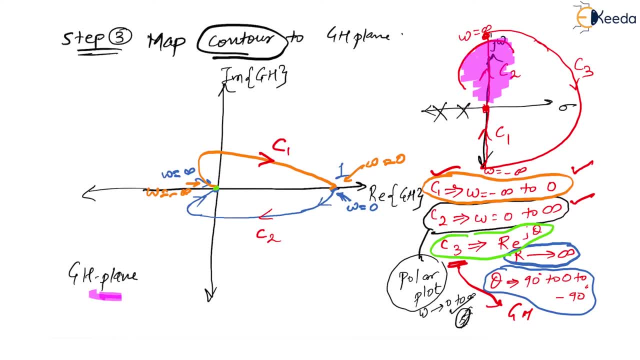 It is 0 in GH plane At some angle: 90 degrees to minus 90 degrees. It is okay, Even if you take other way Round also. Right, We have seen that, Which means it will be mapped in GH. 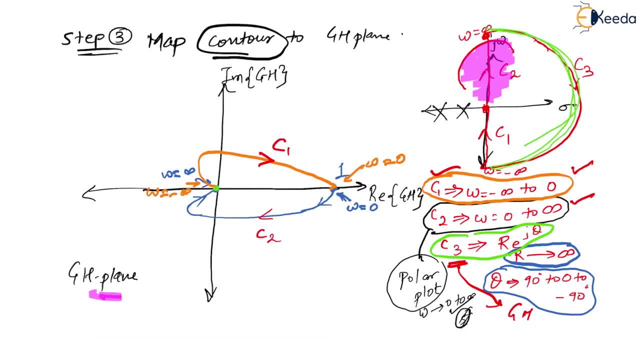 This entire C3 contour, This entire C3 contour which was there. It will be mapped now In terms of a single point At origin. So this is going to be your contour C3.. This is going to be your contour C3.. 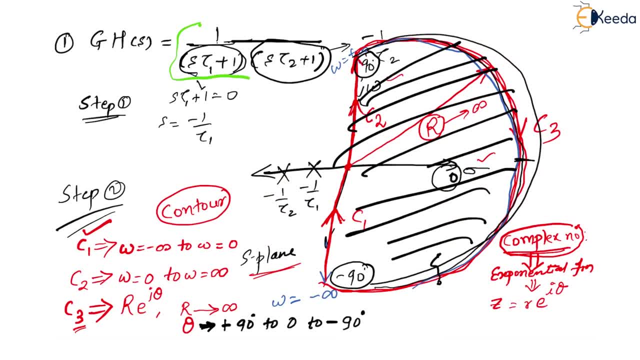 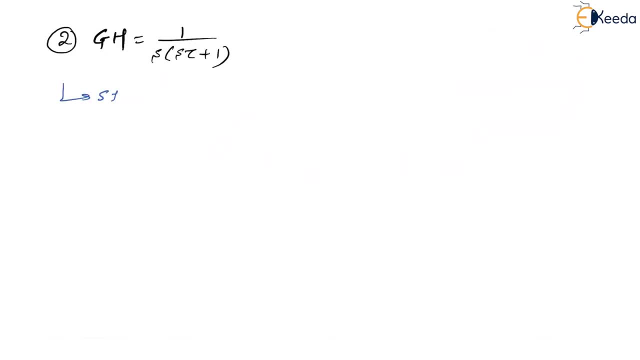 So this ends your Nyquist plot For 1 upon s tau plus 1.. Into s tau plus 1.. Is that correct? Yes, Let us take second example. Yes, So the first step is what? Step 1.? 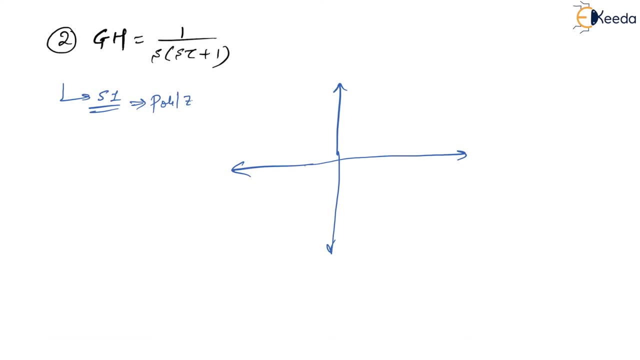 The first step is what To draw the poles and zeros In s plane. Is that right? Yes, So if you see One pole is at origin, So I will draw it here, And another pole is at Minus 1 by tau. 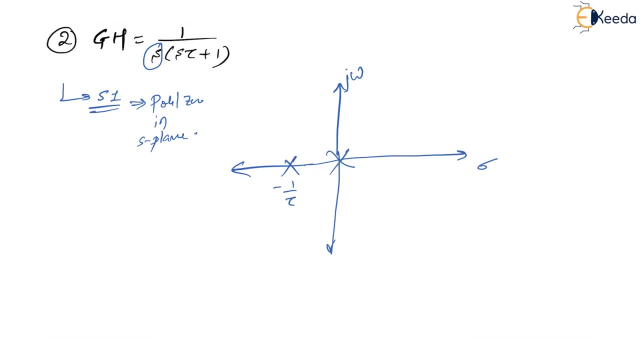 Is that correct? Yes, This is your s plane. Is that correct? Now I am interested in Now step 2.. Step 2 is what? In step 2, we try to find the contours Right. How to find those contours? 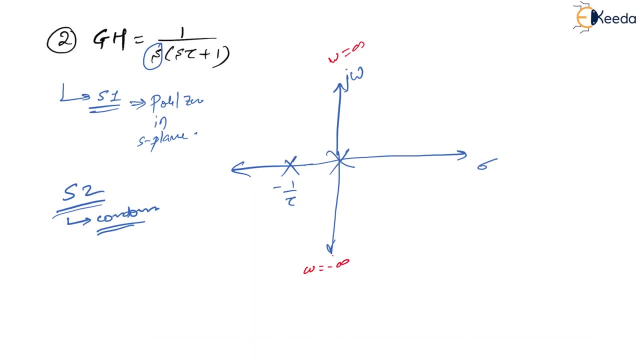 Let us see, If you see it here, From minus infinity. See, this is omega equal to minus infinity And this is omega equal to infinity, Right? C1 is what Omega goes from minus infinity to infinity. Is that right? 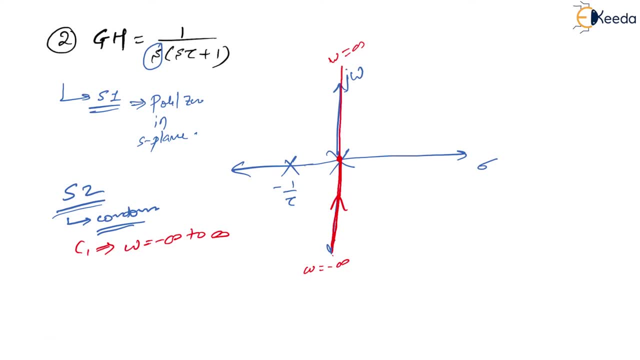 Yes. Now second contour is from where to where? Omega equal to zero to omega equal to infinity. So it is going to be my second contour. So contour C2 is going to be omega equal to zero To infinity. Yes, 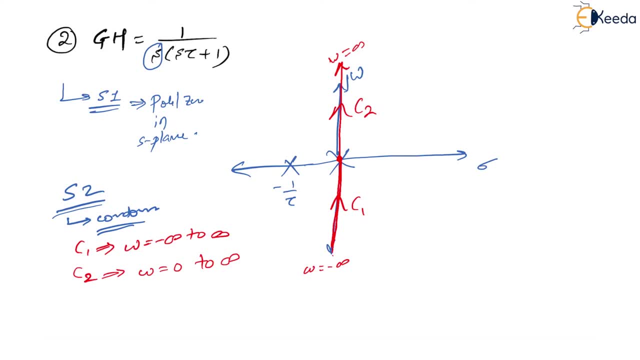 This is going to be contour C2.. This was my contour C1. Now I have to Draw a entire S plane. Now Here you have to understand one thing: What did I say? What did I say, See? 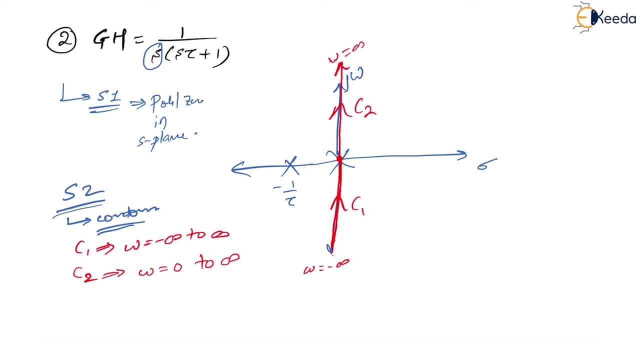 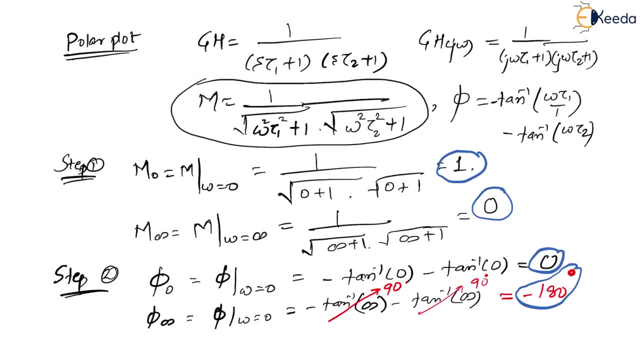 This particular C2 is going to be wrong. I have done it very, very intentionally To show you that students do such mistakes. If you see, If you remember, I have told you one thing: that Bypass Any pole or zero at origin. 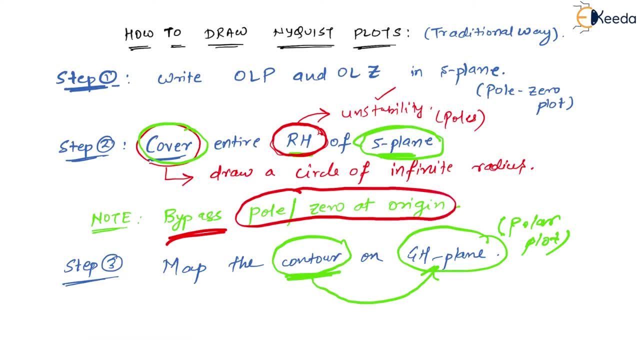 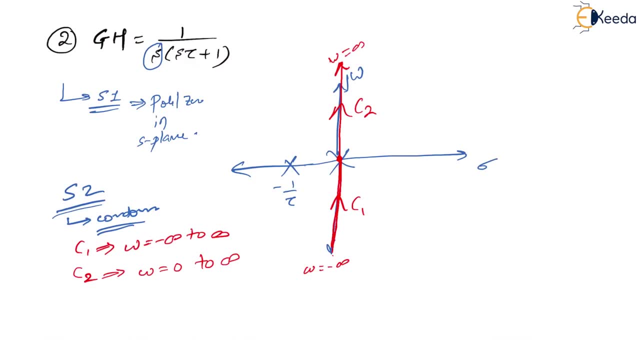 If you remember That I had told you Right That you have to bypass any pole or zero at origin. But If you see, We have drawn this C2 directly. Is it right? No, it is absolutely wrong. So what am I supposed to do now? 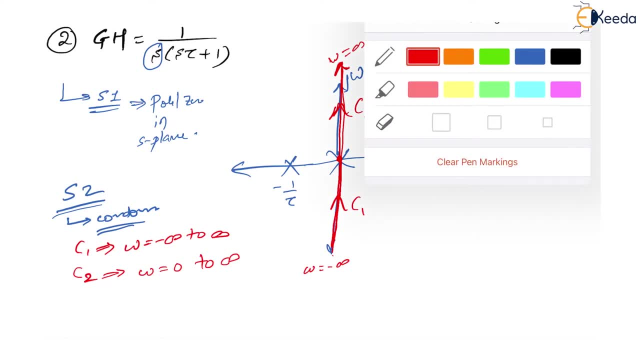 I am supposed to Do it this way. I will show you what, Right Now, This is wrong. Right? We have seen that. How to bypass. Let us see. This is now minus infinity to zero, Right, Yes? 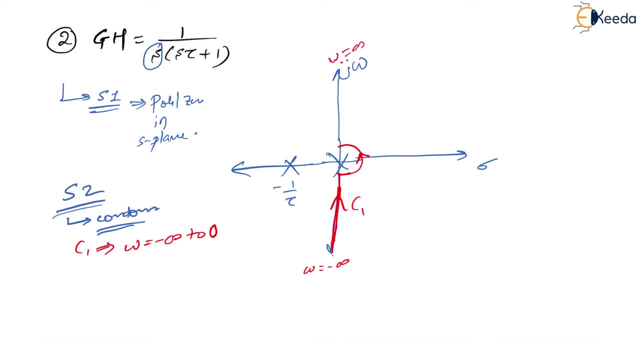 Now, In order to bypass it, You will do just a simple bypass this way And your direction will be this Right, Because you are always starting from minus infinity. So, since it is a contour, Let me call that as C2.. 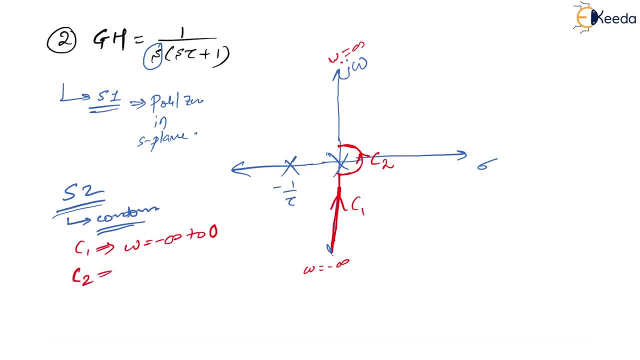 Is that correct? Yes, definitely. Now, if you think of C2.. What is C2 here? What is C2 here? Let us understand This. is very interesting See If you see C2.. Is it a circle or not? 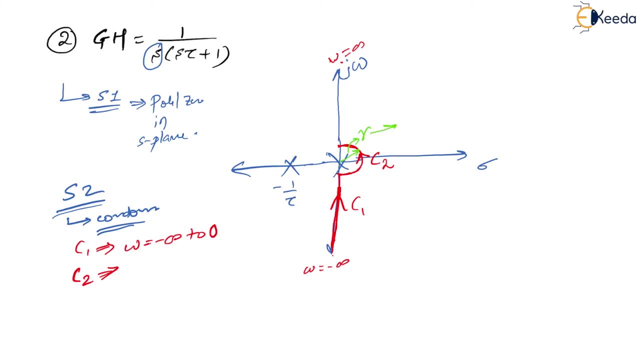 Yes. So what is the radius of this circle? It is tending to zero. It is a very, very, very, very small radius. It is a very small radius, Which means It is tending to zero. So C2 is what? 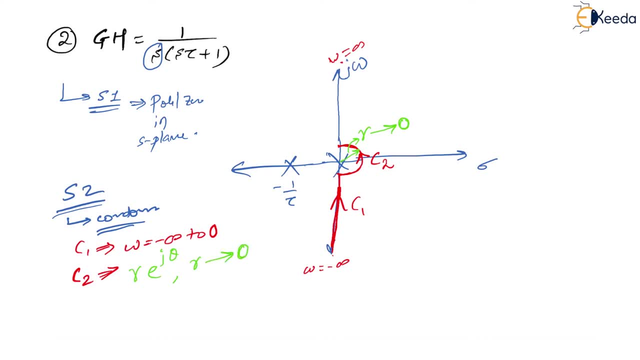 C2 is nothing but r into e, to the power, j theta, Where r tends to zero. I hope This point is very, very clear to you. Now, angle: What about the angle? See, If you see, this is zero degrees. 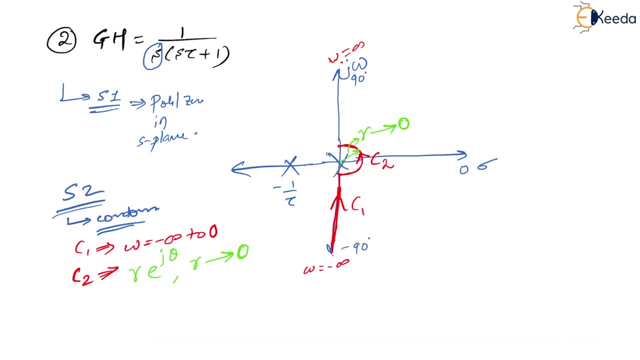 Then this is plus ninety degrees, Then this is minus ninety degrees Right Now. If you see, I am moving in this direction. If you see C2 direction, It is from minus ninety degrees to zero And then again to plus ninety degrees. 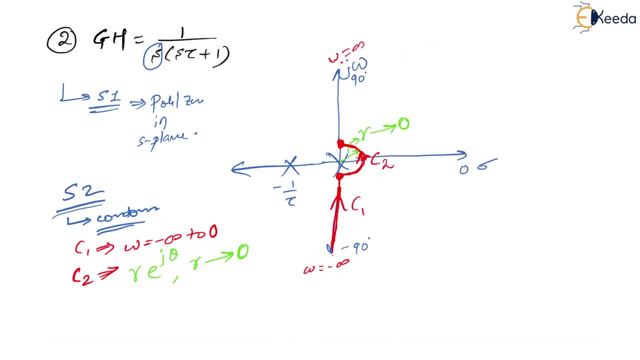 Is that right? See Again, It is from where to where: Minus ninety to zero And again plus ninety, Which means theta varies from where to where. It varies from Minus ninety degrees To zero To plus ninety degrees. 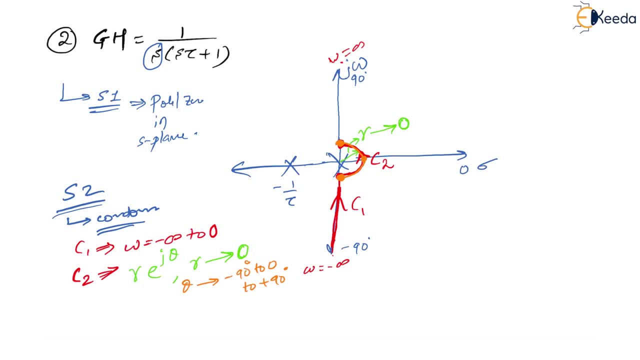 I hope this point is very, very clear to you Right Now. If you think of contour C3. Contour C3 will be where C3 will be from again, zero to, Because- see now Student may ask me, Sir, but it is not exactly equal to zero. 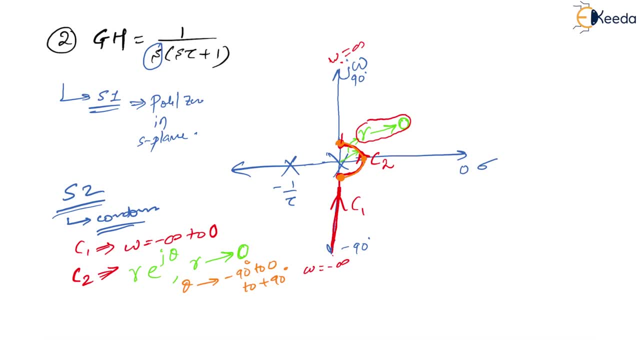 Yes, I know, It is very, very close to zero, Which means it is very, very close to zero- Not exactly zero, But it is very, very close to zero. Right? So I can say that even this is zero. So this goes from zero to positive infinity. 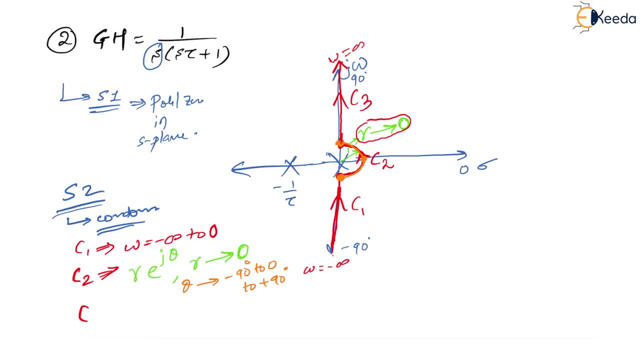 And this is contour C3.. So what is C3?? C3 is what C3 is what It is: a contour Where omega varies from zero to infinity. Is that clear? Yes, Now What about C4?? Is there any other contour left? 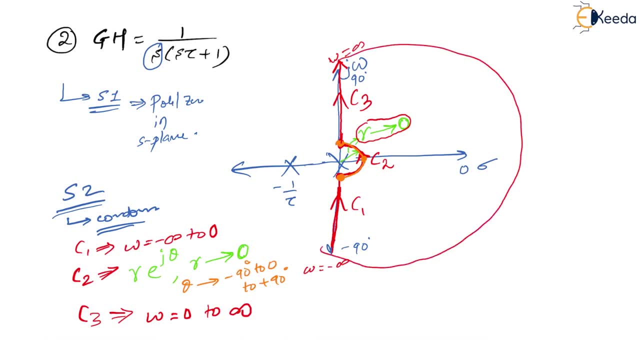 Yes, Because you have to cover this entire right half of S plane also, Which means you need to have- You need to have one more contour, Which is C4.. What is that contour C4?? As usual, we know that it is also going to be. 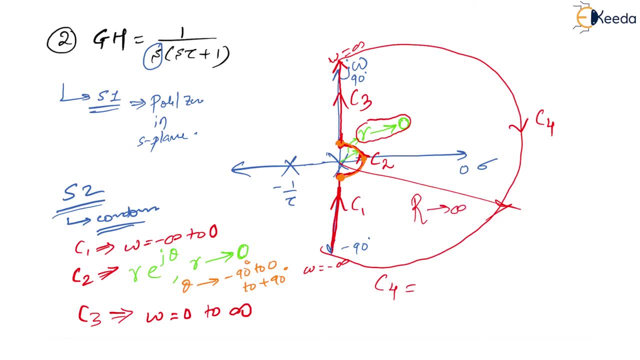 Because that radius is going to be R, This radius is going to be capital R, Which tends to infinity. So it is going to be what? C4. Where R tends to infinity. And what are the angles? The angle, if you see the direction, is this way: 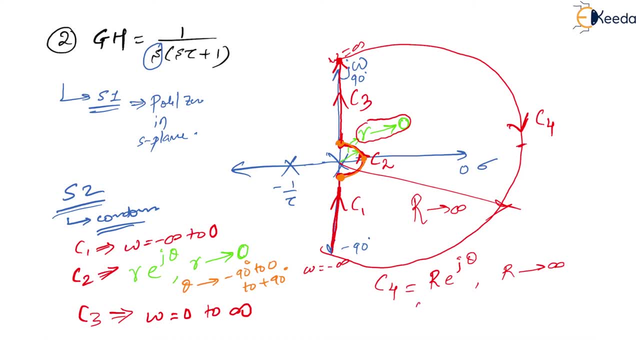 Which means it is starting from plus 90 degrees to zero And then again to minus 90 degrees, Which means theta varies from. Theta varies from where to where. It varies from 90 degrees To zero degrees, To minus 90 degrees. 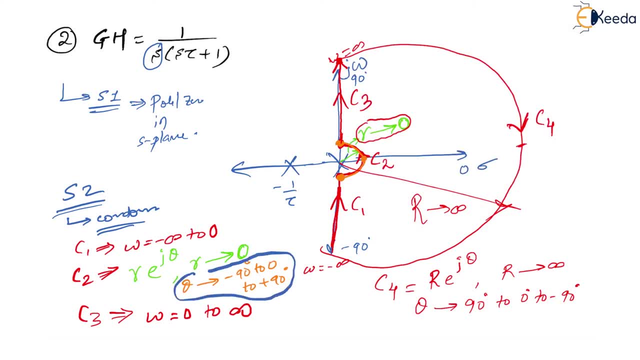 If you see, if you observe, Here theta varies. This small theta varies from Minus 90 degrees to zero To positive 90 degrees, Whereas here theta varies from Positive 90 degrees to zero to minus 90 degrees. I hope you are understanding this point. 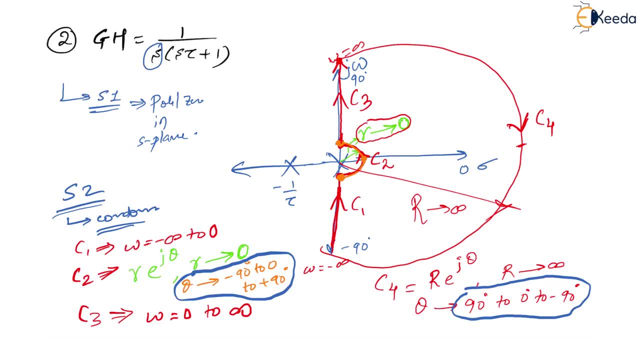 These are very, very small, small points. So it is very, very important. Now, next, Let us see how to map all these From S plane to GH plane. Let us see that. So if you see, if you just see, Your C3 contour is what 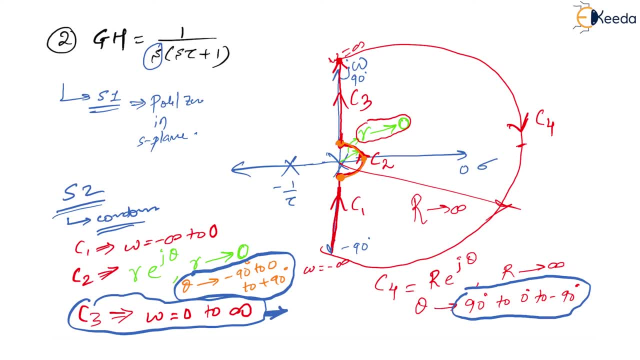 It is from omega, which is equal to Zero, to infinity. It is nothing but what. It is nothing but what Polar plot. So let me draw the polar plot. If you remember, we have taken this question, GH equal to 1 upon S into S, tau plus 1.. 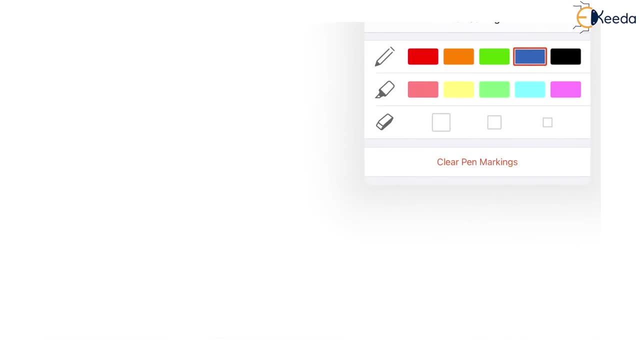 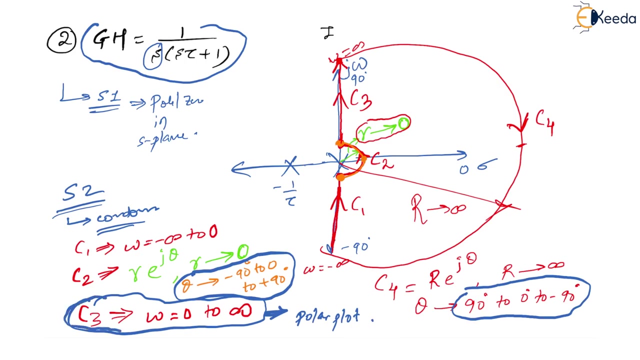 So I already know the plot for this. So the plot is going to be how much? See, This is real part of GH And this is imaginary part. Imaginary part of GH. Okay, Yes, Contour C3, which is from omega equal to zero to infinity. 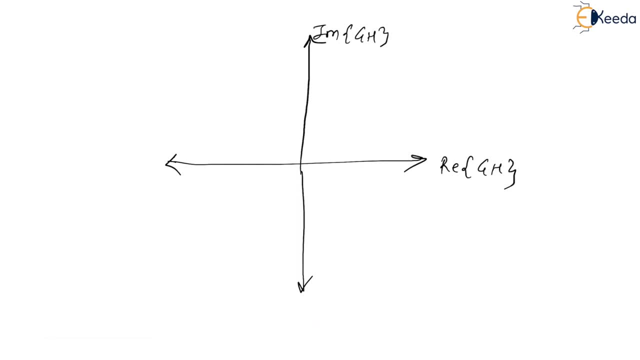 Is nothing but the polar plot, Right? So the plot for this? we know that It is going to be from here to here. We have done N number of examples on this, So I hope that you all know How to draw a polar plot. 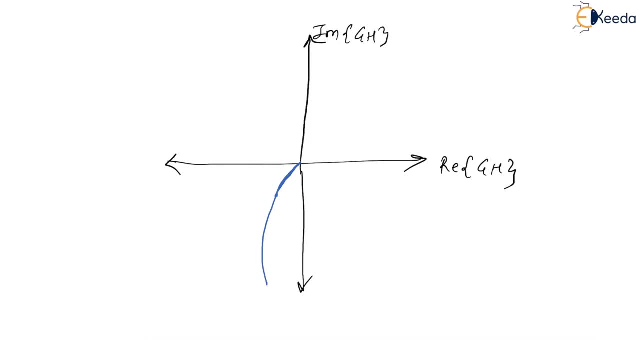 Because Now we are interested in finding out The Nyquist plot. You already know how to draw a plot. Now we are interested in finding out How to draw a Nyquist plot. I hope it is very, very clear. So this is going to be omega equal to zero. 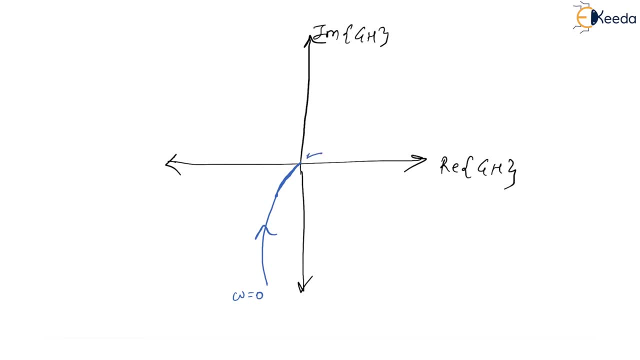 It is going to start here And this is going to be omega equal to infinity. Is that correct? Omega equal to infinity? And this is the polar plot. And what is the contour? This is representing contour C, C3.. This is representing contour C3. 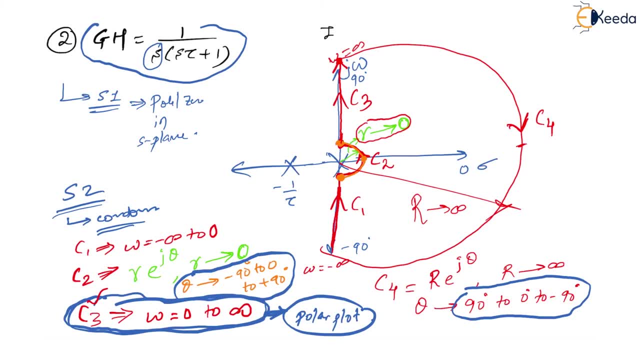 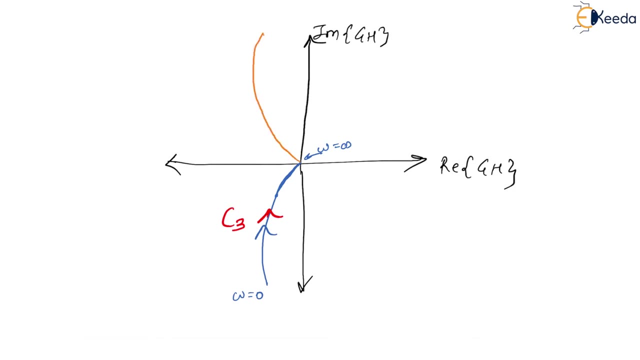 Is that correct? Yes, One battle is done Because of C1 contour. C1 contour is what? Omega equal to minus, infinity to zero, Which means exactly reverse. So I am going to have a mirror image here this way, So this becomes: 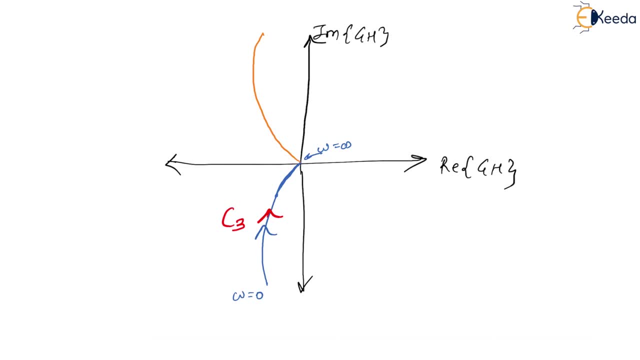 One Right. So this is another one Which is this way. Now, always remember Nyquist, plots are always continuous in nature, Are always Continuous in nature. Why? Because if you see, Always, the direction has to be followed, You cannot keep that this. 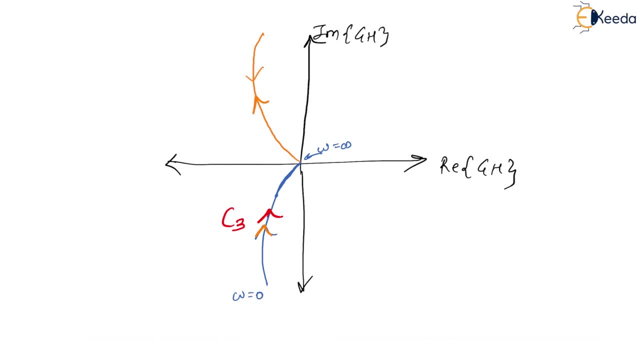 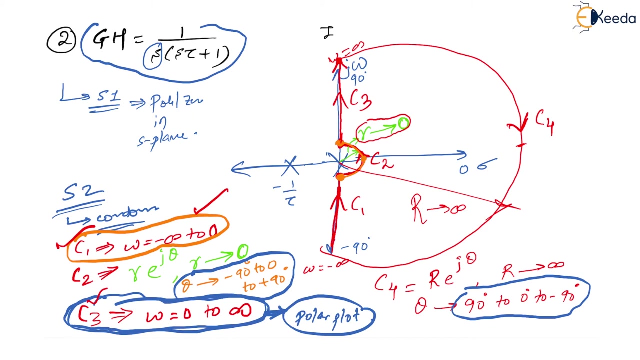 As you know, upwards and this To be downwards. You cannot do that. This is very, very wrong. And if you see, It is showing you contour C1. Right, So this is showing contour C1. So C3 is done. 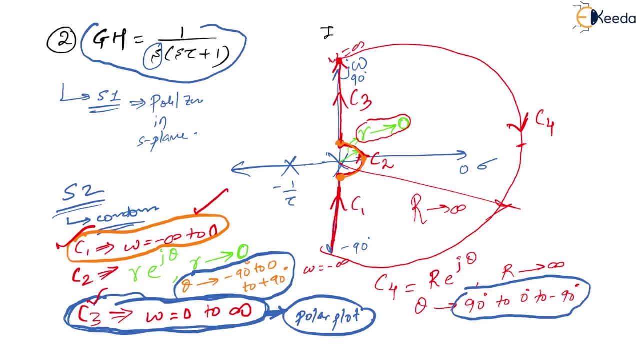 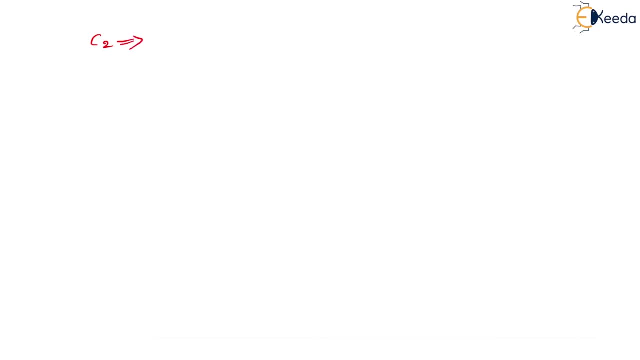 And C1 is done. Now I am interested in C2.. How to draw C2?? Let us see that. What was your C2?? C2 was nothing but R into e, to the power j theta, Whereas this was small r right. 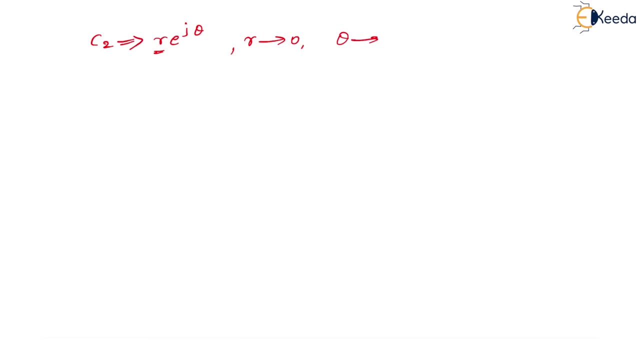 And we saw that r tends to zero. And this theta which is there, It is varying from where to where. It is varying from minus ninety degrees to zero To positive ninety degrees. I hope you all know this Right Now. if you see that again, yes, 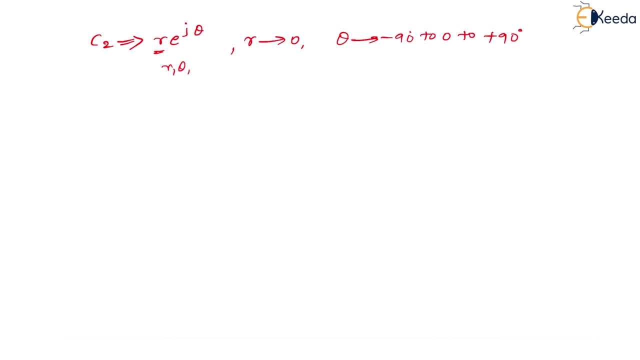 R and theta are the variables, So let me just do so. So if I just Replace them in gh, If you remember, Our gh was what Gh was? one upon s Into s tau plus one Right. This was our gh. 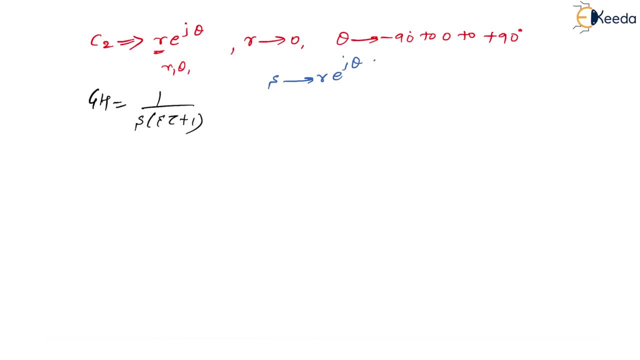 Now, if I replace R into e to the power j theta, What do I get then? I get gh of R into e to the power j theta, Which is equal to one upon R into e to the power j theta Multiplied by. 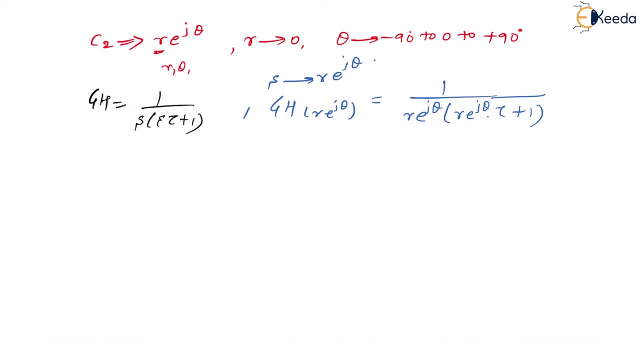 R into e to the power, j theta Into tau plus one. Is that correct? Yes, Now we know that. We know that R tends to zero. Yes, r tends to zero. Which means what? How much is the magnitude? How much is the magnitude? 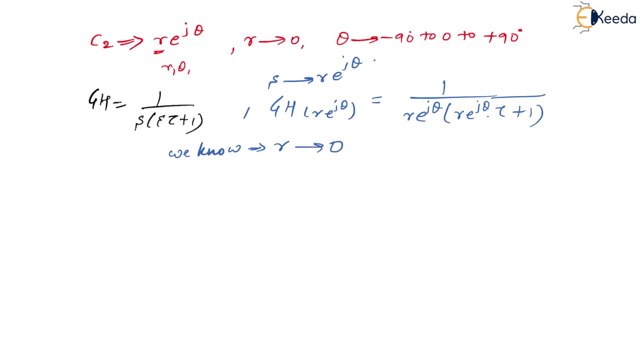 Let us find So for that, If you know that Mathematics, You have Already learnt that, In such a cases, while applying limits- Because this is nothing but limit, As r tends to zero One by r into e, to the power j, theta. 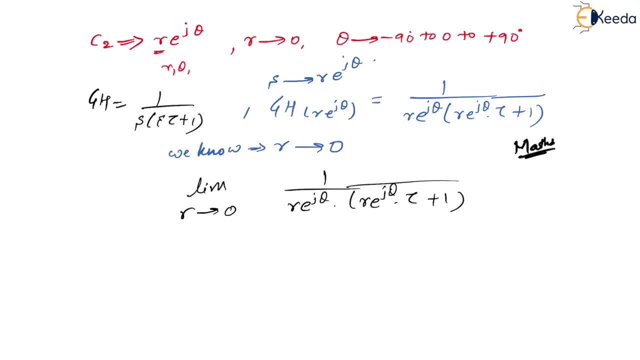 Multiplied by r into e to the power, j, theta Into tau plus one. So you have seen that This particular term Can be made zero. Here you can put r, R equal to zero. What you are left with is Limit, as r tends to zero. 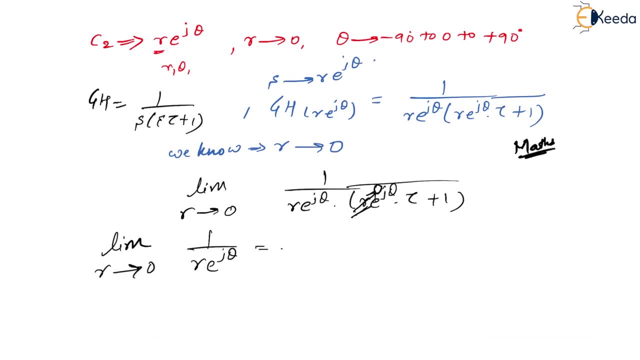 You have got this one upon r into e to the power, j theta Right. So if I can show it this way also, That it is limit, as r tends to zero, Which is nothing but One by r into e to the power. 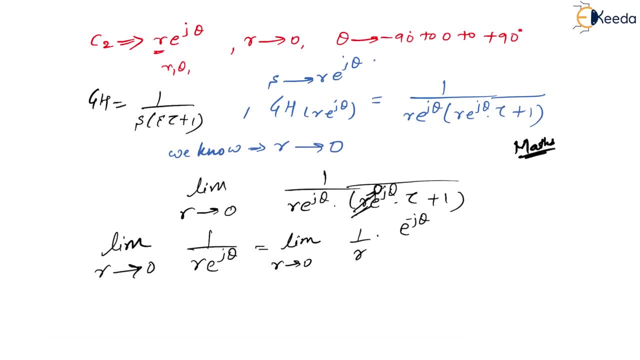 Minus j theta, Yes. So now this indicates what. This indicates that your magnitude is this Limit, as r tends to zero. This is your magnitude, one by r And Angle is what? Because of this minus, If you see, 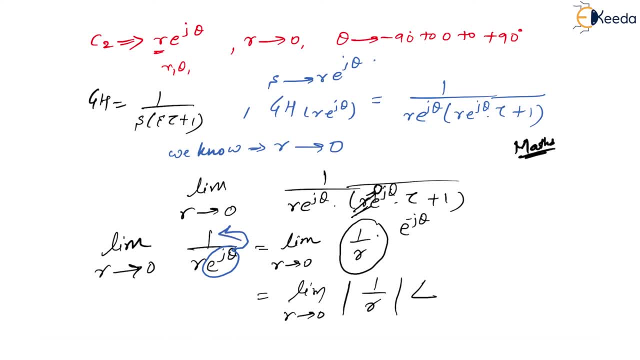 When your e to the power j theta Goes on the top, This sign changes to minus j theta, Which means Now I am going to have this angle to be minus theta. This is nothing but the polar form. Already you have learnt it in mathematics. 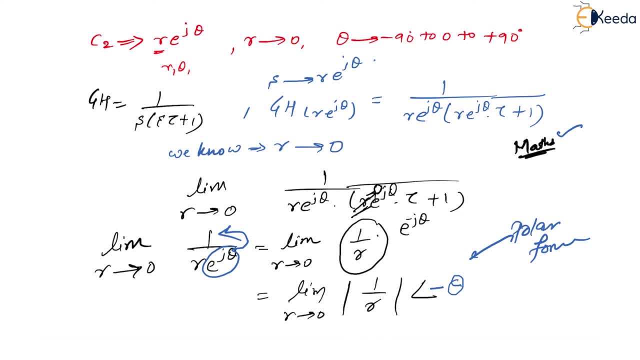 Right, Yes. Now see it here. If you put r Tending to zero, What you get? You get one by zero. So you get magnitude to be equal to infinity, Right, Yes. And if you see, What about the angle? 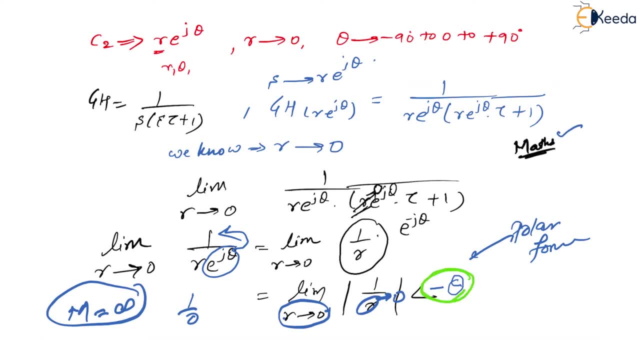 Just see This angle is minus theta. It means that In your s plane Your theta was varying from minus ninety to plus ninety, But now in gh plane, Your theta is going to vary from Plus ninety degrees To zero To minus ninety degrees. 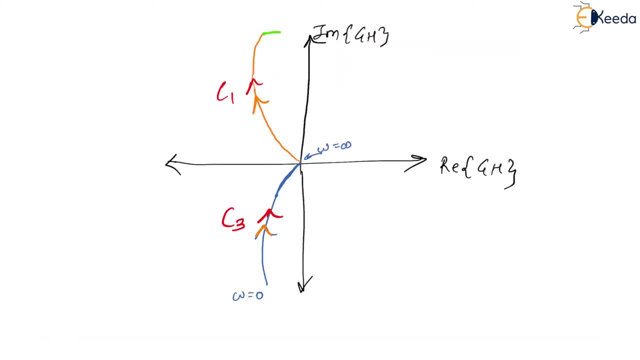 I hope you are understanding this point Right. So if you see Plus ninety degrees To zero, To minus ninety degrees Is what has to be the travel cell, And if you see How much is the radius, Then the radius is going to be infinity. 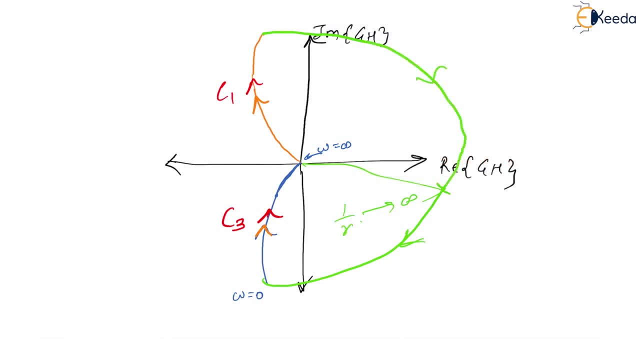 I hope you are understanding this point Right. So if you see The angle of one by r Tending to infinity, I hope it is very, very clear, Right? Yes, Now Rather, I can show it this way also. 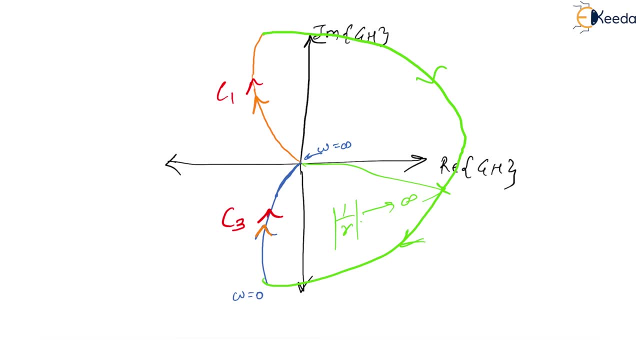 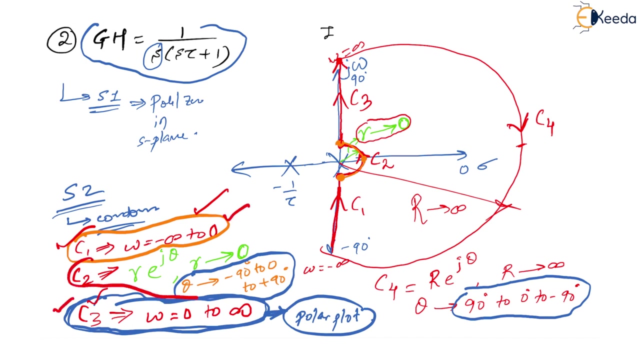 Mod of one by r Tending to infinity Right. Yes, Now see it here. What about? You have successfully plotted c1.. You have successfully mapped c3. And you have successfully now mapped C2 as well. So c2 is also done. 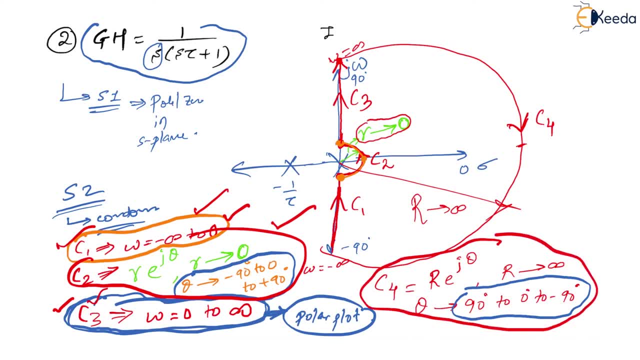 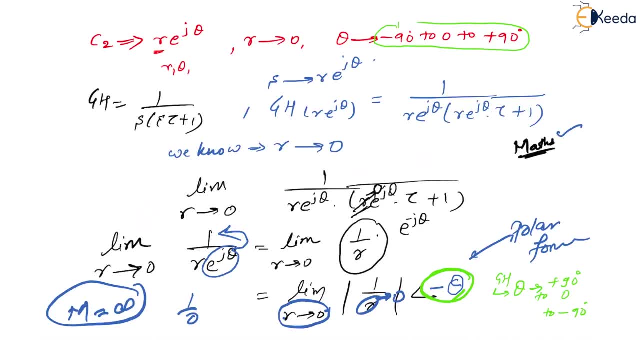 Now how to map c4.. How to map c4.. Let us see that C4 is what r into e to the power j theta Right. So If you see c4. C4 is what r into e to the power j theta. 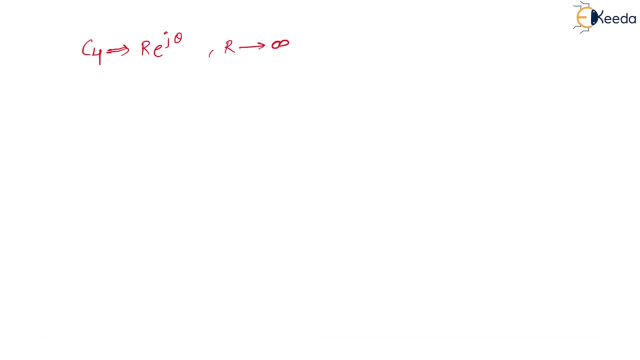 Where r tends to infinity Right Now. yes, similarly, If you just think of, What you have is gh. gh is equal to what 1 upon s into s tau Plus 1.. So, yes, similarly, you have to find gh of. 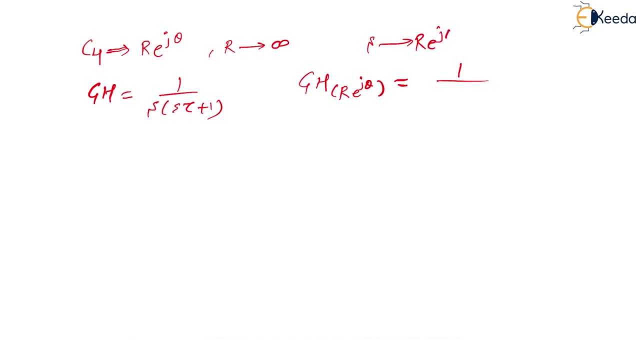 r into e to the power j theta, Which means you please put s as r into e to the power j theta. If I put it to be j theta, r into e to the power j theta, What I get is r into e to the power j theta. 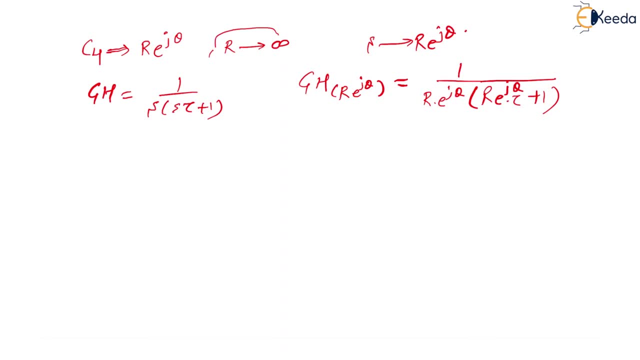 Multiplied by r into e, to the power j, theta Plus 1. is that right? Yes, now you know that r is tending to infinity, Which means this becomes infinity, This becomes infinity, So, which means it is nothing but 1 by infinity.